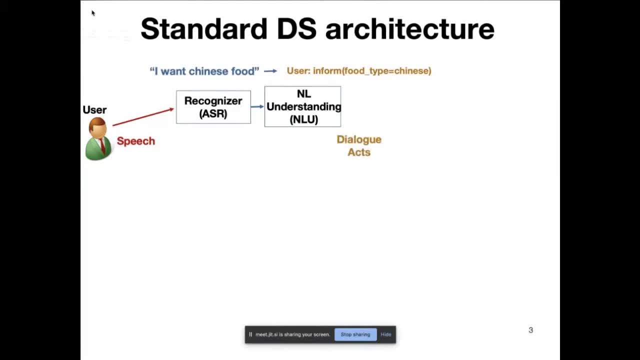 food would be one type of semantic representation. So those things are usually called dialogue acts, sometimes called intents, user intentions- And they are then fed into a component called the dialogue manager. Dialogue manager typically has access to a website or resources on the web And it has to do a couple of things. It has to figure 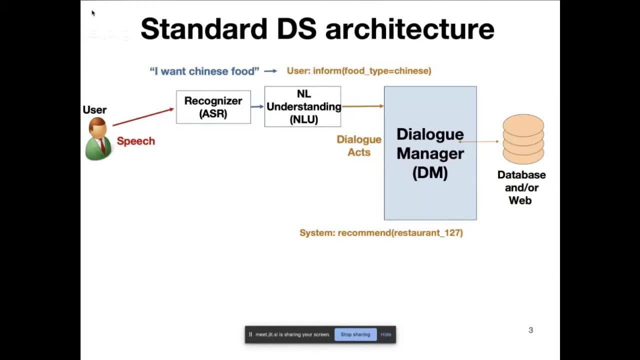 out what it is that the user is doing in the context of the whole dialogue so far, And then it has to hopefully think of a response. So in this case it's going to do a response that says: I recommend a particular restaurant. Now, again, that's also a dialogue, that's. 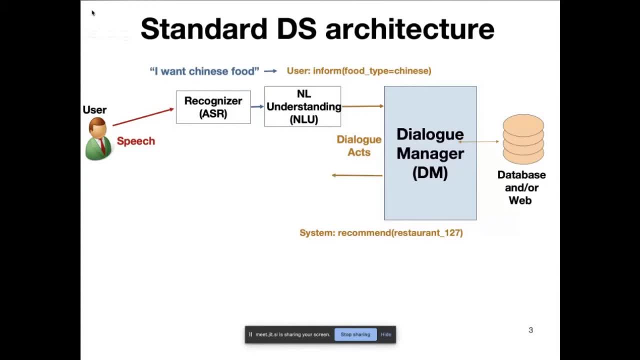 a dialogue act. It's not natural language yet, So it has to be fed into a component called the natural language generator And that effectively decodes dialogue acts into strings of words. If you go to a speech synthesizer and you might get an output like that, where 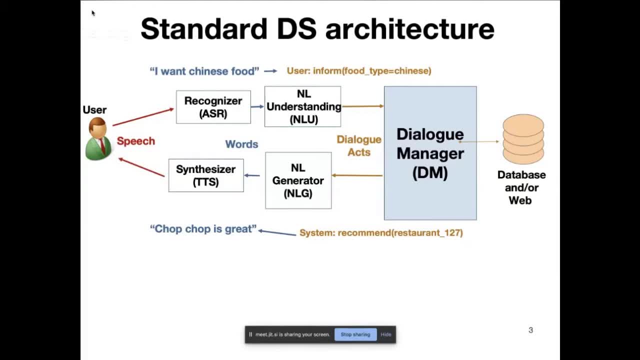 number 127 is chop, chop And we tell the user: that's a great restaurant. So that's a great restaurant. So that's just the way that spoken dialogue systems have been built, probably for about the past 15 years or so, And what's happened more very recently is that some of 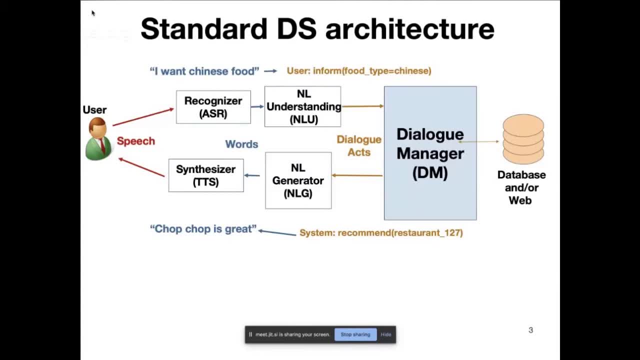 these components have been by deep learn methods And I'll talk about those later. So an important point when you're dealing with robots Is that the output is not only speech synthesis, but it's also the robot: maybe moving, pointing, having facial expressions, maybe have an animated face. So an important thing for Spring and 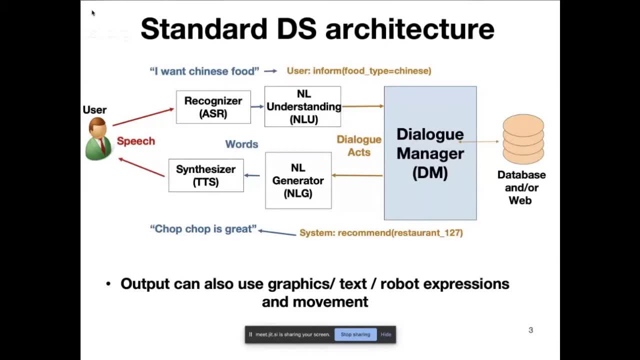 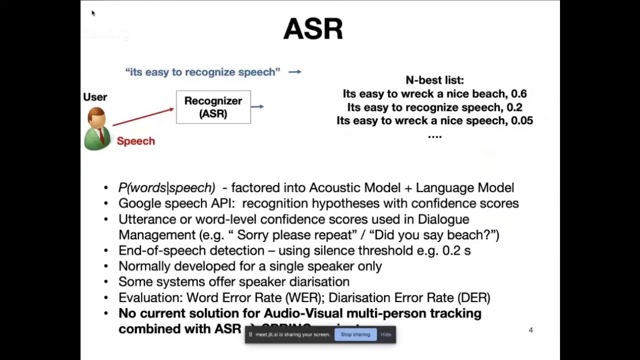 in all these projects with human robot interaction is how the robot output can be used to communicate as well as just speech. Okay, So I'm going to quickly go through each of those components, Just very briefly describing them and some of the methods that we use and what I think the challenges, or 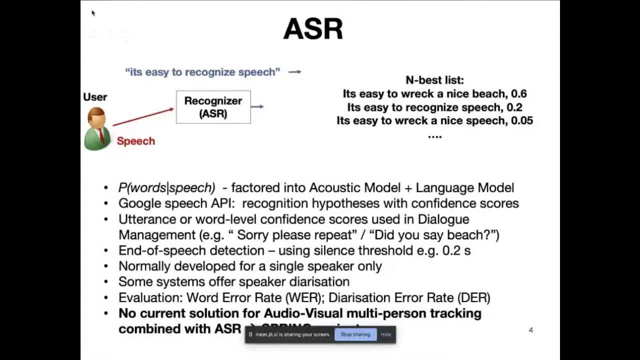 interesting problems we have are in the Spring project. So with speech recognition- ASR is automatic speech recognition- We have obviously this component which is trying to decode audio into strings of words, So someone might say it's easy to recognise speech. and 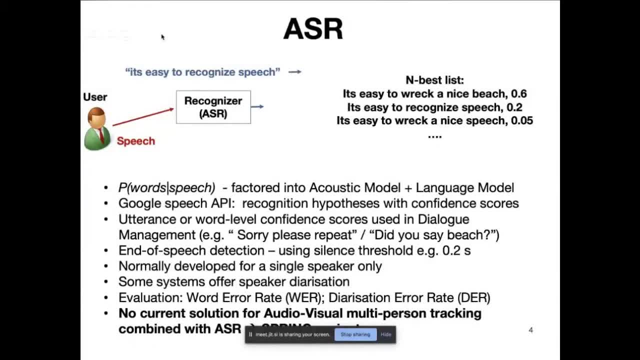 then typically in a modern speech, recogniser, you get an end best list hypothesis of what the user really said with some confidence scores. So the numbers on the right are these numbers. here I hope you can see my pointer. those are the key numbers. So this is the number. 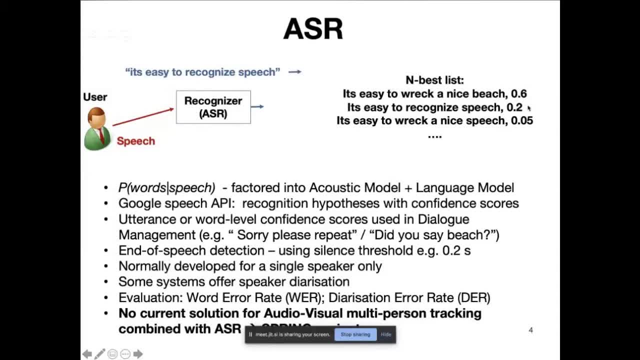 of words. Okay, confidence scores uh from the recognizer. so you can see that. you know there are many different ways that uh recognizer might decode some speech and some of them are correct and some of them are incorrect. so i mean, there's a huge, massive literature on how to build speech recognizers. 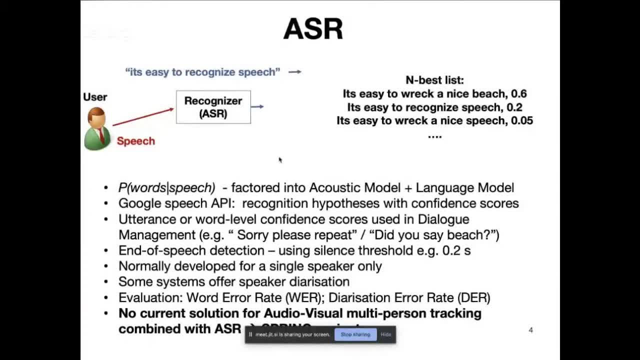 effectively. the way it's done is you: you split the problem into acoustic modeling and language modeling and um. what we typically use in our systems nowadays is the google speech api, which gives us these kind of recognition hypotheses along with confidence scores, and it's important for us in dialogue management to use the confidence scores um so that we can, for example, 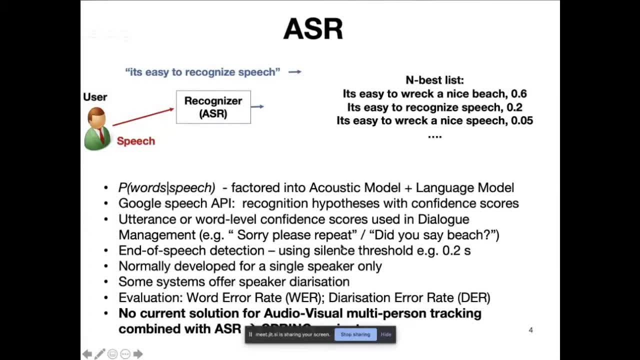 uh, say things like: oh, please can you repeat that? if we were not very confident about the whole utterance, or if we were, it was a particular word we didn't hear very well, we could, we could clarify. you know, did you say beach or did you say speech, um, so we can use those. 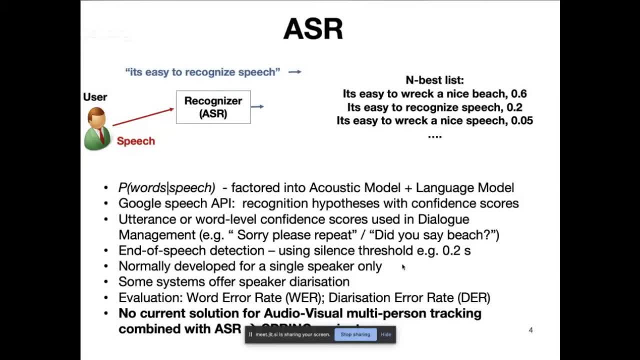 consequences. sorry, sorry, oliver, can i interrupt you? yes, please. so yeah, this is very interesting, but i uh, do you have a confidence score per word or for the whole phrase? um, it depends on the particular speech recognizer that you're using, using um. so with google speech, api, i think we actually get word based confidence scores. 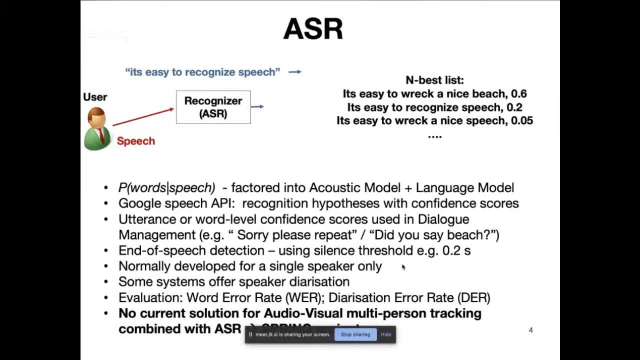 um, we certainly have had word based confidence scores from different recognizers in the past. okay, um, i think. i think google speech does give word based um. okay, so then, uh, we like to use those confidence scores in in dialogue management. there's also a very important point, which is when we detect the end of a user's speech. so typically you set a. 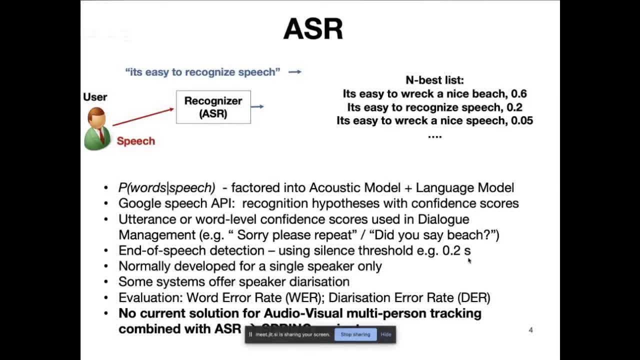 silence threshold, so maybe 0.2 of a second. this can actually cause problems because in real life, for example, we put a robot into a supermarket and we found that real people often pause quite a lot in the middle of what they're saying and the speech recognizer can think that they're. 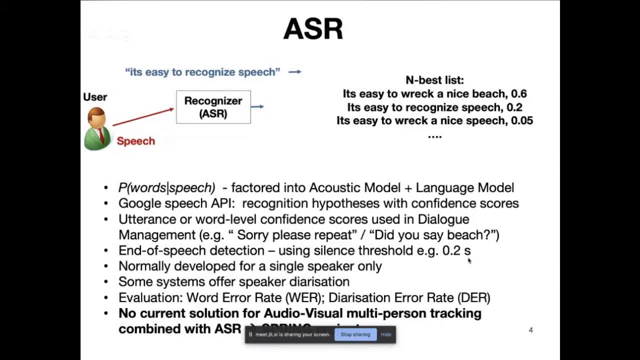 finished speaking when, in fact, they're just pausing um. so this is something that's quite challenging in real world situations and when we have multiple people speaking, this is going to be even more important to deal with. um. so we have experimented with language modeling methods for. 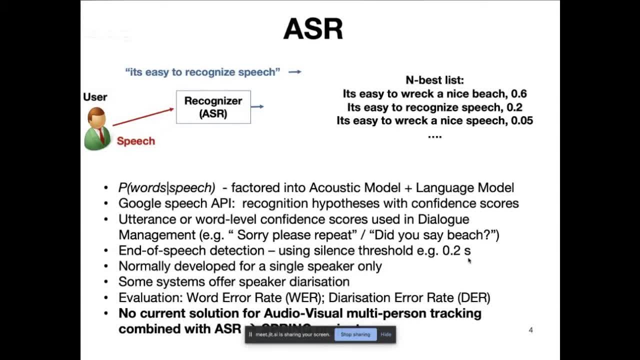 detecting end of speech, and that might be something we need to do. so another point to note is that, you know, most speech recognizers are developed for a single speaker at one time. sorry, there's a lot of noise, somebody needs to mute, okay? um, these systems develop for a single speaker only typically, and um, we have the problem. 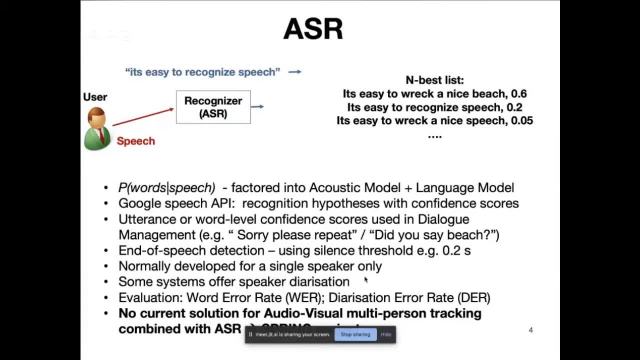 hello, sorry, is it possible to ask a question? yeah, if someone speaks, let's say continuously: so till the pause of 1.0.1 second. there is no feedback from the recognizer. well, um, it depends again on what which recognizer you're using. some of them produce um in real time. 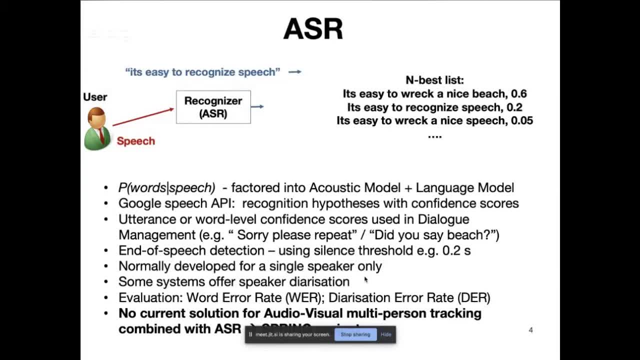 hypotheses, you know, in incremental uh hypotheses as the person is speaking um. so yes, you can, you can get immediate um word by word hypotheses. okay, what's provide google api for? i think google api just gives you um incremental word by word hypothesis as the person is speaking. and what is the latency of the the? 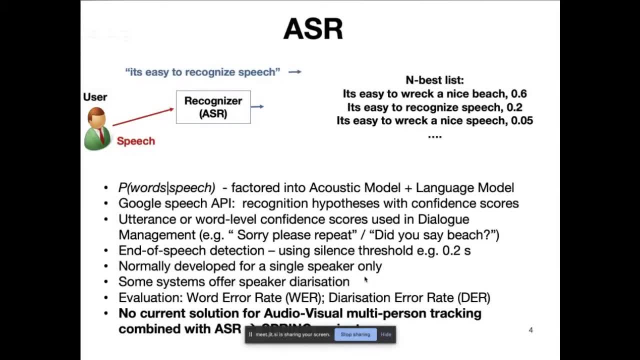 once google api is being sent the the speech, how long it takes google api to return the interpretation of the speech? yeah, that's a very good question and that is something we've had problems with in the past. um, it's a you know, because it's been doing cloud-based speech. 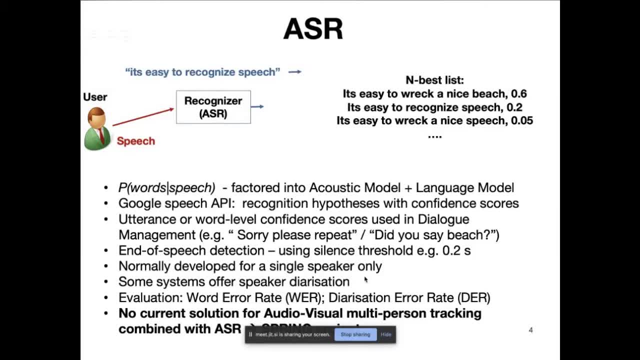 recognition. you can have a time lag, unfortunately, so that's a good point. it's obviously much better to have a recognizer that's locally um installed on or embedded on a device so that you don't have a big time lag with network connections. so that's a very good point. we we would ideally have a local embedded speech recognition so that 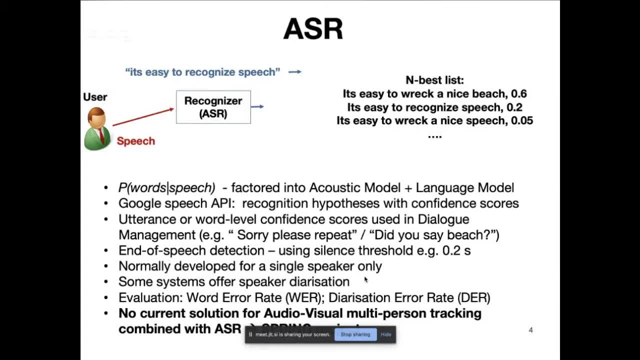 we can have very fast uh interaction with the speech recognizer. can i just say, um, from experience, the governmental results is uh under a second, depending on your. can you repeat the figure? what is the latency? again, it's, it's, it's um, well, under a second normally, depending on your internet speed. uh for the incremental updates, but the incremental updates. 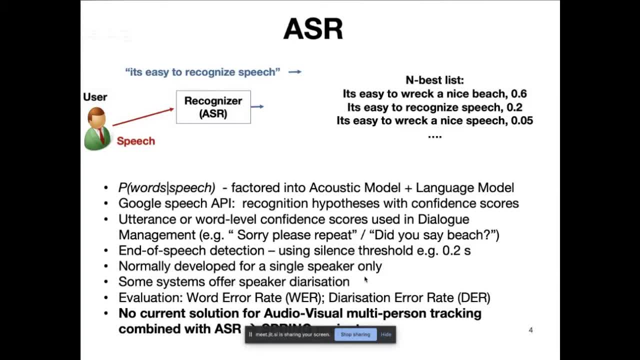 are less correct than the final update and there is timing issues, as oliver said. so that's something we will have to look out for in the project. yeah, so i i didn't hear the figure. can you repeat the figure again please? under: he says: well, under a second. 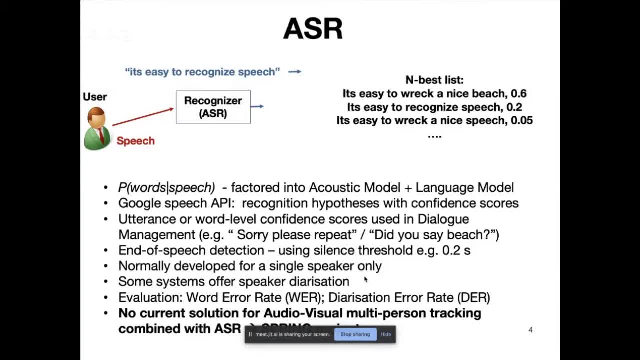 um, yeah, so it's under under one second is the normal latency. um, but even that is quite annoying. yes, even that can be quite bad. um, because this is too huge lag and it is not, i would say, natural speech if i'm talking with in a phone and the latency is more than 1.2 seconds. 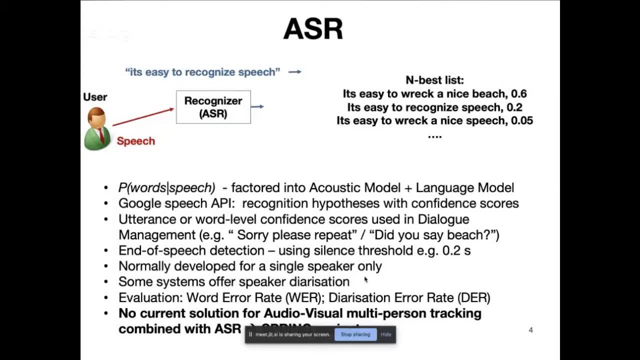 it's considered a quite annoying discussion. yes, i totally agree. i mean, this is one of the interesting things is that we're quite far away from com, real, true, fluid, fluent, conversational speech because of these time lagging issues. um, so i i think anything that can be done to bring the latency down. 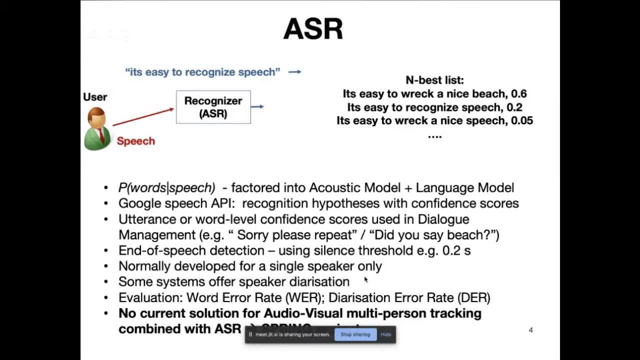 will really help these kind of systems, but with cloud-based solutions at the moment, you know, having a latency of 10 to 15 seconds. if you switch to a system where you have just one at hand, zu of under one second is probably state of the art. 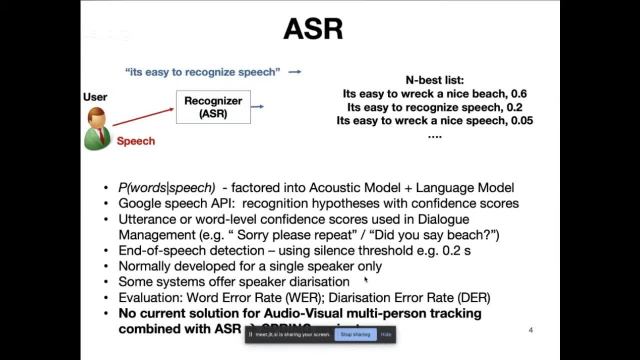 But embedded solutions are really going to be more important in the future. So, for example, the new Google Pixel 4 phone has the speech recognition all embedded within the phone itself rather than cloud-based, And it's devices like that that I think are going to drive much faster speech interaction. 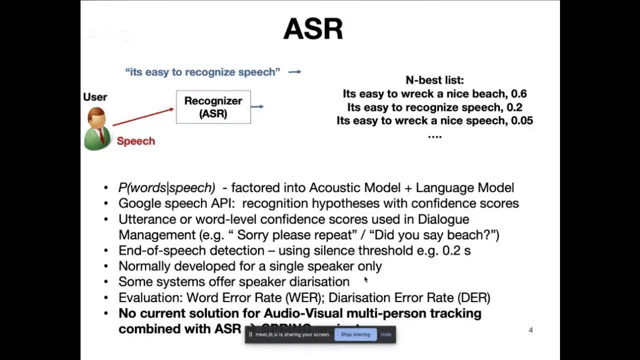 Sorry, but I think that this latency, there are two kinds of latency, right, It's the intrinsic latency of the speech recognizer itself and the latency due to the fact that you are sending a request to a cloud, right? So the intrinsic latency. 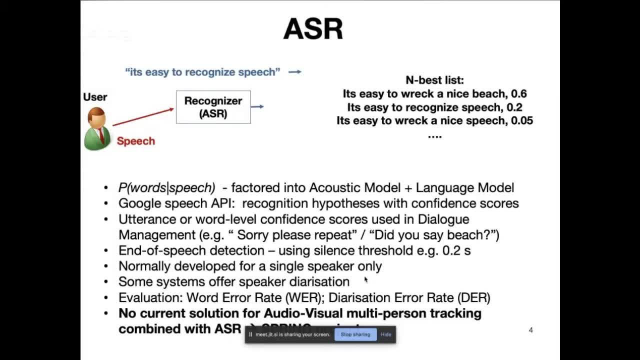 The latency of the ASR is not an issue anymore, if I understand well JOHN MUELLER- I think that's pretty much true. I mean, I don't know the numbers, but the latency we're getting is mostly due to network traffic. 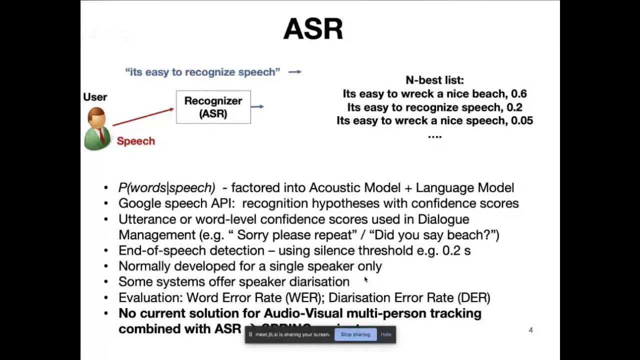 OK, thank you, JOHN MUELLER- OK, so good. So, obviously, I mean it's important to measure the accuracy of a speech recognizer. It's typically done with what's called the word error rate, And that's something which we'll have to pay attention to. 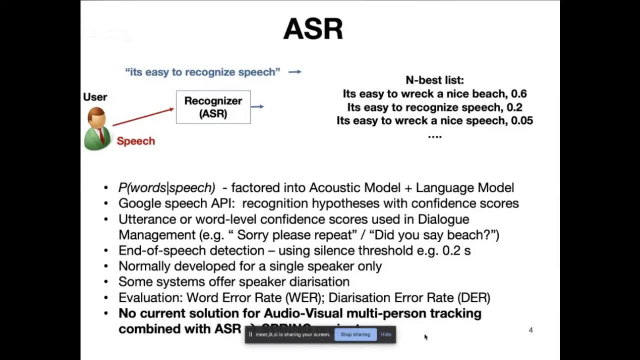 and together with the diarization error rate. So I think the challenge, as far as I understand, for Spring. I mean, I've been looking into this. I haven't found anybody who's combined audio-visual multi-person tracking with speech. 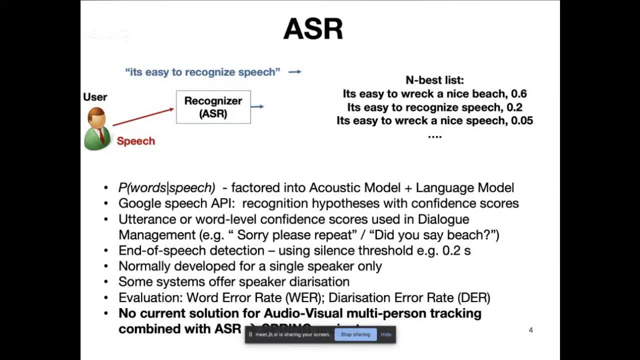 recognition, And I think it's really important to be able to do that, Because obviously, what we want to do is be able to hopefully accurately, in real time, find out the words that particular different people are saying in a social situation. So I think, as I've said before, I 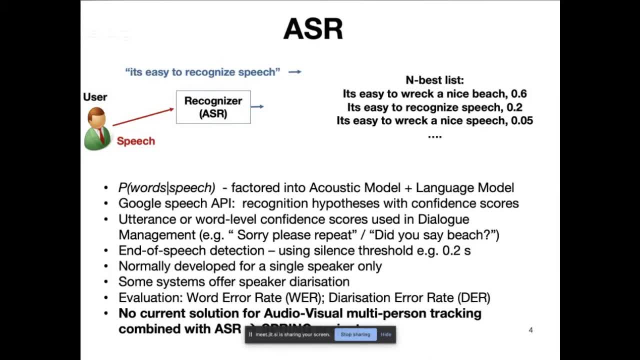 think there's a really exciting opportunity in the project to try and work on that problem And it's really fundamental. I mean, if we want to model multiple people interacting with a robot, we kind of have to have some reasonable solution to this problem. 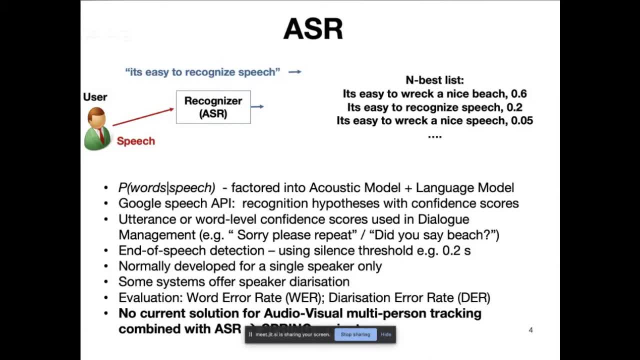 Sorry, Oliver, to interrupt your grind, but I fully agree with this And, in fact, I think that this is something that we are taking very seriously, And I hope that the next couple of months I will try to come up with some of our students. 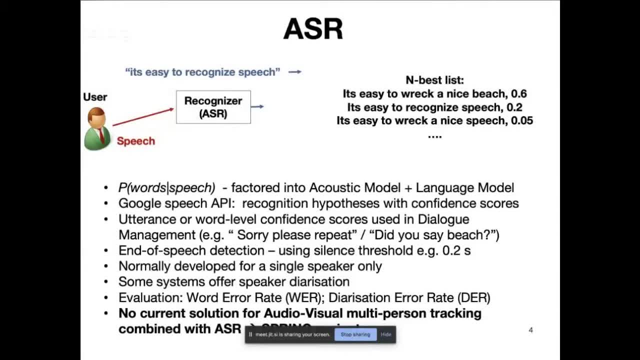 to, let's say, at least on paper, some kind of a solution. Yes, basically integrates ASR into our current audio-visual tracker. so basically that we can we're able to assign, basically to send to an ASR signals, let's say a temporal segment that correspond to a single person. yes, 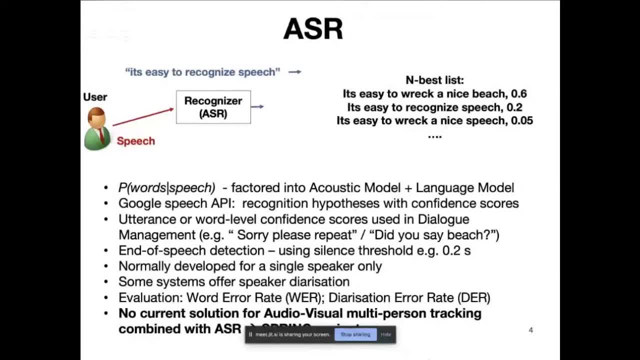 yes, that's, that's great and we're very keen to collaborate on that. okay, great, yes, yeah, the reason for which I'm asking this: world recognition versus phrase recognition is very important because sometimes, when you our experience that when you have multiple people chatting, sometimes this segment of speech that 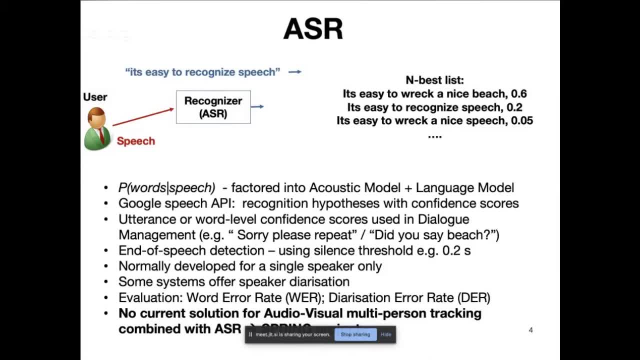 you are sending to Google. Google speech does not correspond to a phrase that you are sending to Google. Google speech does not correspond to a phrase that actually makes sense from a semantic point of view. right, so you should solve this issue. yeah, sorry, a beam former should solve this issue. okay, we can, yeah. 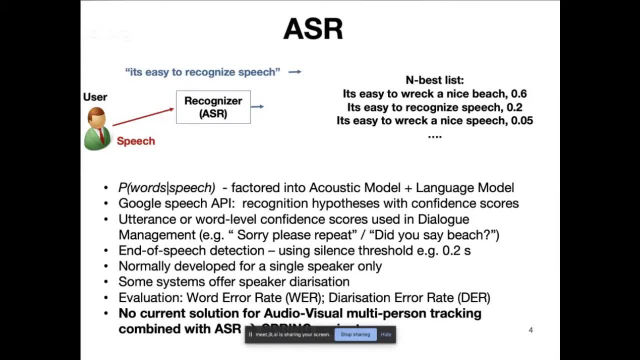 we can. yeah, yeah, I think that we should put a speech enhancement or be forming in the pipeline somewhere. yeah, I agree, okay, but I mean, as you said, it's also related to the language modeling issue, because your language, you, the language model, has to be able to detect fragments of speech that are not 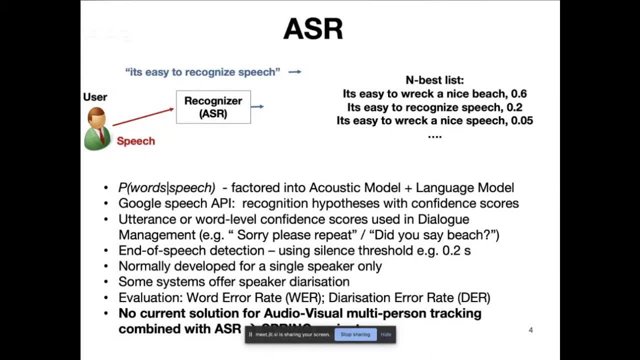 necessarily complete sentences or utterances. exactly, yeah, so I think there is something interesting there about having a language model that is trained on fragments of speech rather than full utterances. so, yeah, there's a huge amount of really interesting things to do here. okay, sorry, I will let you talk now because, yeah, I'm on slide four and it's. 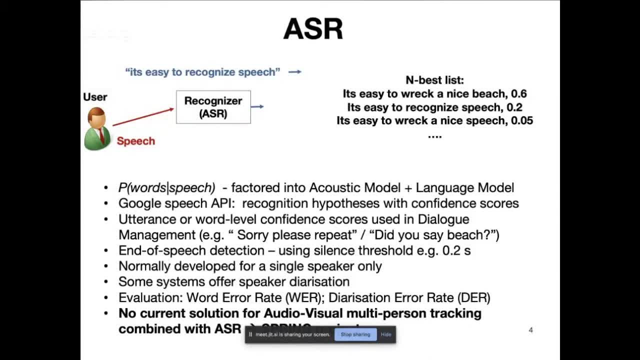 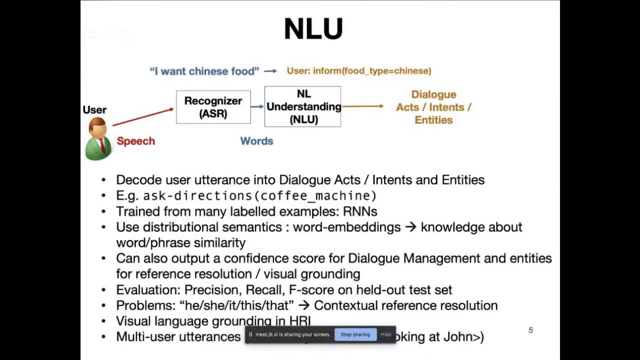 20 past 10, so okay. so natural language understanding is obviously next key component. we need to decode the recognized speech into dialogue acts or intents and entities. so an example might be: you know, I want to ask for directions to the coffee machine. this might be something that happens in the spring. 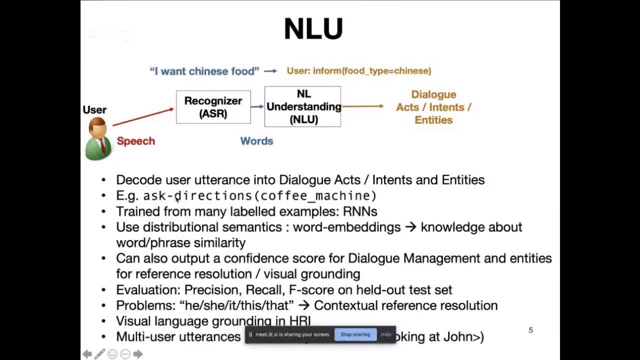 project. so there's an entity which is the coffee machine and the dialogue act, where the intent of the user is to ask for directions. So, basically, in modern AI, these systems are trained from many, many labeled examples, using different types of recurrent neural networks. 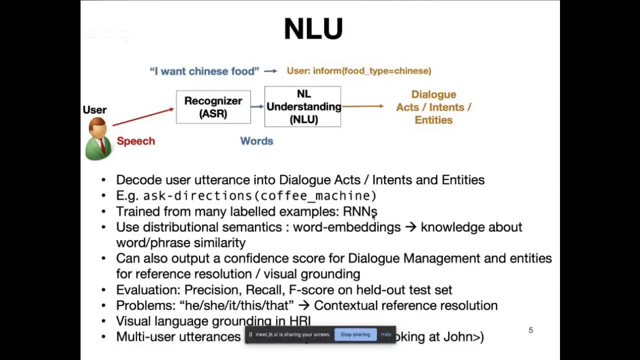 And in addition, they use distributional semantics. So that's the idea that we can look at word similarity by saying that words with similar meanings appear in similar contexts, And so we're able to rapidly build language understanding components effectively using pre-trained word embedding models. 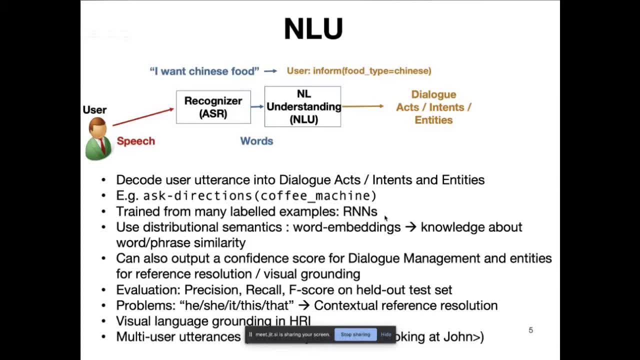 So there's lots of powerful techniques now that are doing data-driven approaches to this natural language understanding problem. In addition, we can get a confidence score for dialogue management, similar to the data-driven approach to language understanding, And we can also pull out entities that the person is talking about, and that's important. 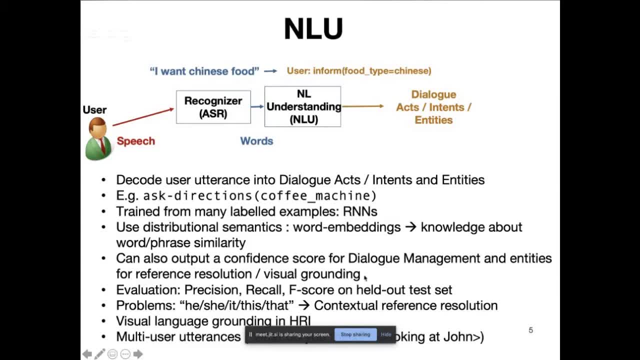 for reference, resolution and visual grounding. So if somebody talks about a particular entity like the coffee machine, we might actually have a visual or spatial location of that object. So that's something that we can look at in the context that we want to deal with. 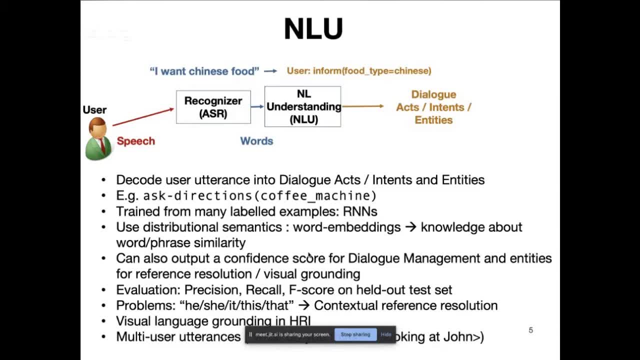 So these systems are then evaluated using metrics like precision, recall and F-score on a held-out test set. So typically you have a development set of examples. You have a different set of examples that you use to test the accuracy of the language. 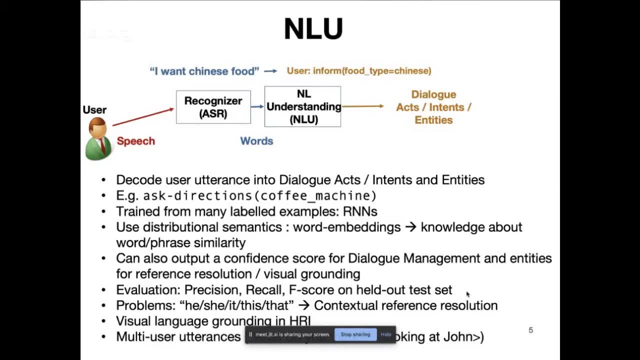 understanding component And there's lots of interesting problems still to deal with. For example, when someone says you know he, she, it, This or that, We have to understand in context what they're talking about And that's why we have the dialogue history as part of the system. 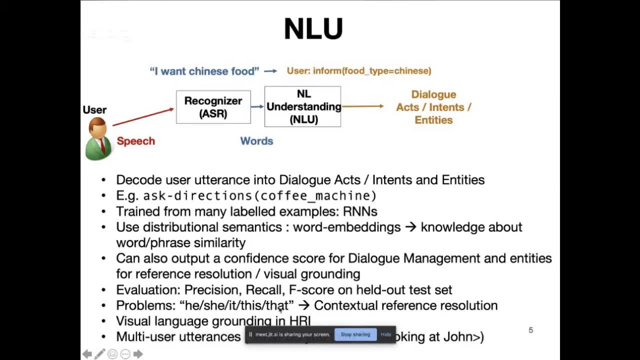 So we can try to understand what people mean by these expressions. Also in the project we have visual language grounding issues, So I know that's part of the spring project as well- Trying to Map entities that people are talking about onto spatial or visual representations. 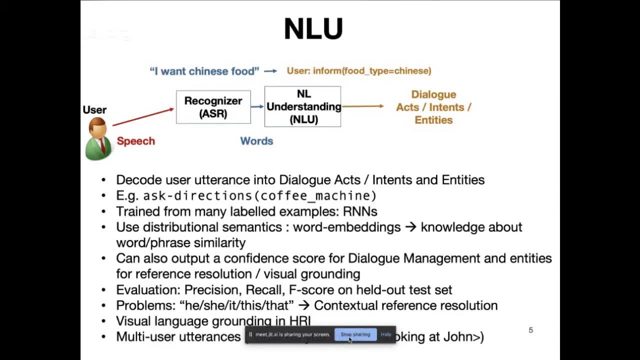 And actually I'm not sure if you can see the final bullet point, But the If you click hide, I think it will help. Do I hide? Can I hide this thing? Yeah, if you click hide, yeah, Oops. 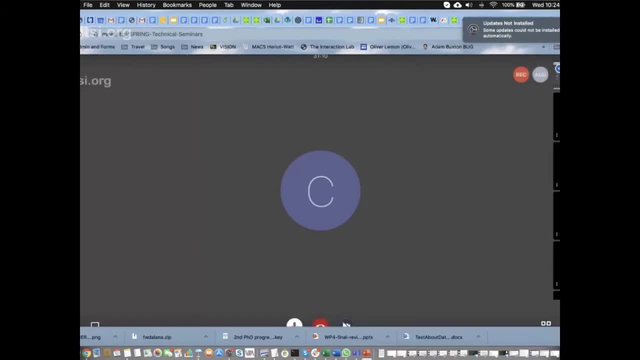 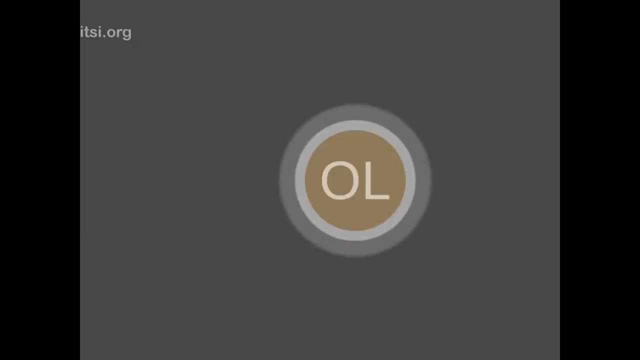 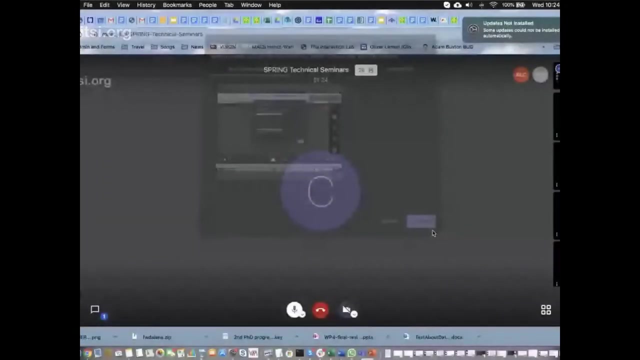 Perfect. Oh no, Is that working? Oh, we don't see your slides anymore. Yes, exactly, We lost your screen. Yeah, I know, So it won't. That didn't work. Let me do that again. I'll just go back to where I was. 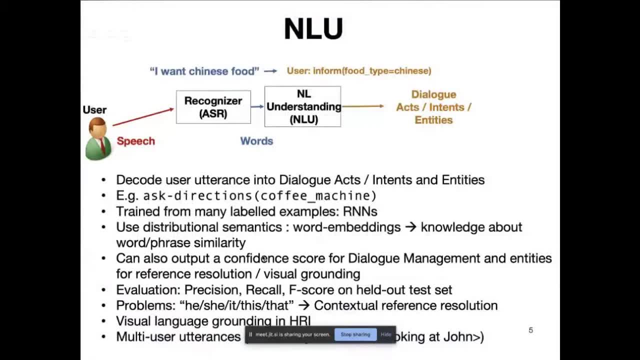 Okay. So what that final bullet says is that multi-user utterances are really interesting in spring. So, for example, if I say what do you think- And I'm looking at John- Then this means I want to know what John thinks. 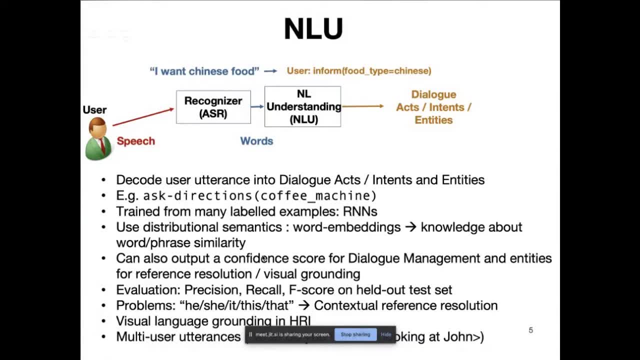 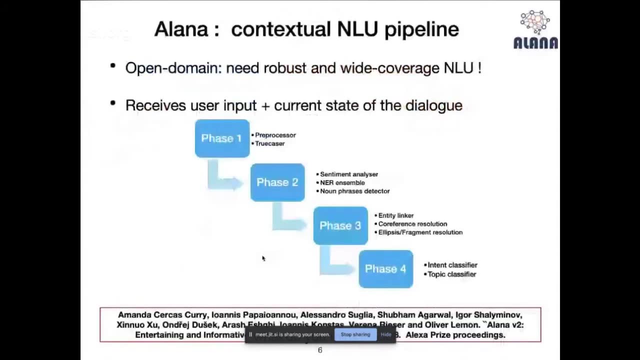 And so there's a very interesting multimodal aspect of language understanding here. where we're looking at, We care about the gaze of the person speaking as well as what they said, So that's really interesting for spring. Yeah, Sorry to interrupt you again. 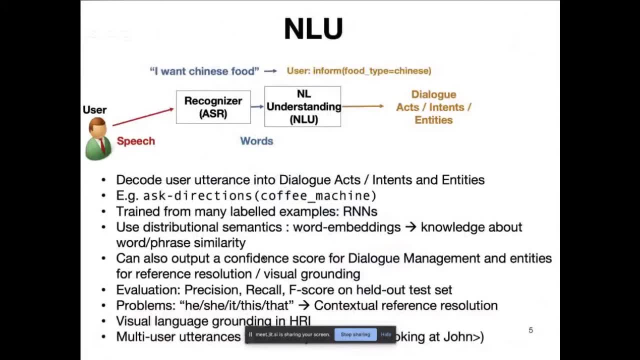 But indeed I also recognize this as a very interesting thing. So maybe in- I don't, I don't know- In a forthcoming seminar I can give a talk on what we Our work on tracking the visual focus of attention of people. 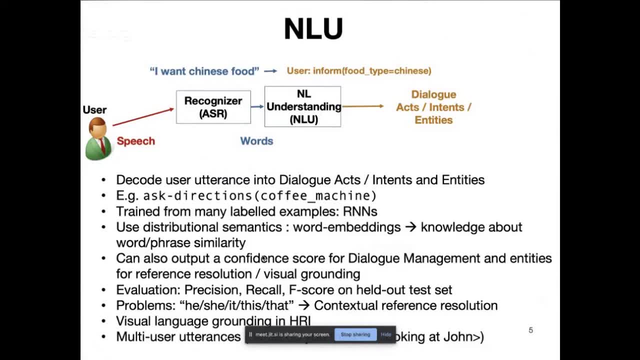 So yeah. So just to mention that, this is something also that we have looked at, And I think it's very relevant to integrate this into Yeah, Yeah, Yeah, Okay. So I think that would be a kind of socially intelligent natural language. 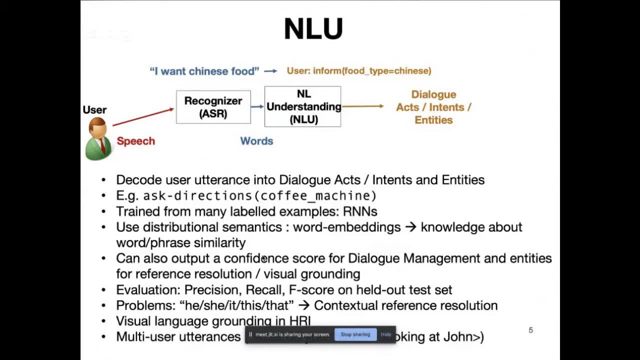 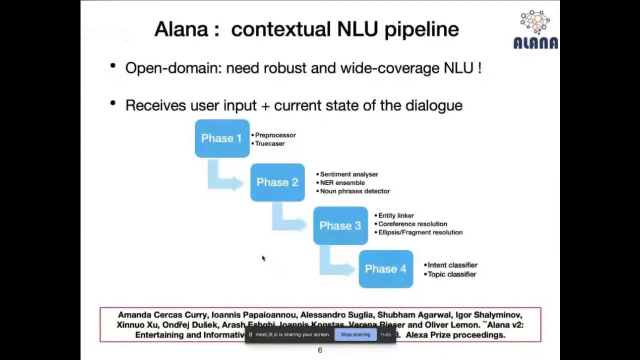 Language understanding or something which I don't think. Again, it's something that, as far as I'm aware, nobody has done that. Okay, So just to very briefly talk about the Alana system, the natural language understanding that happens there. 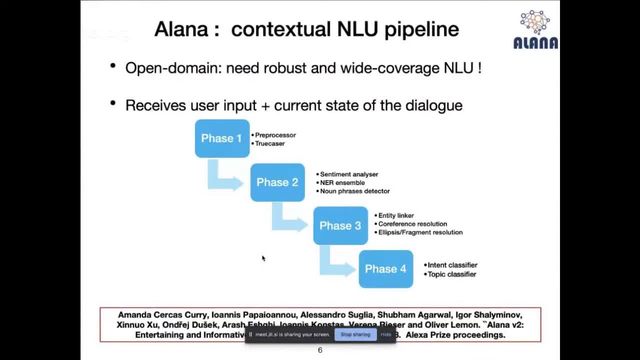 We have a really rich language understanding component which is effectively able to pull out even sentiment of what the user is saying, as well as the noun phrases, the named entities, And do this kind of a resolution of co-reference. So if I say you know I like him, it's able to figure out that him is somebody that I'm speaking about earlier in the conversation. 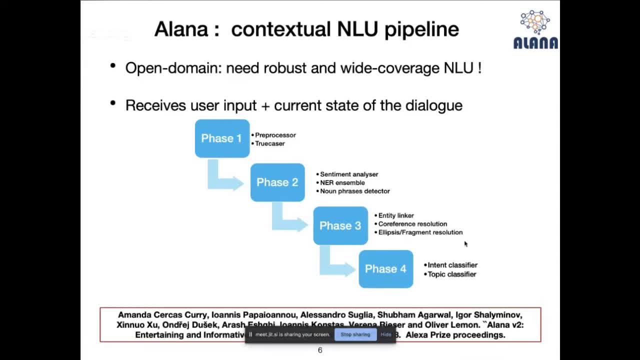 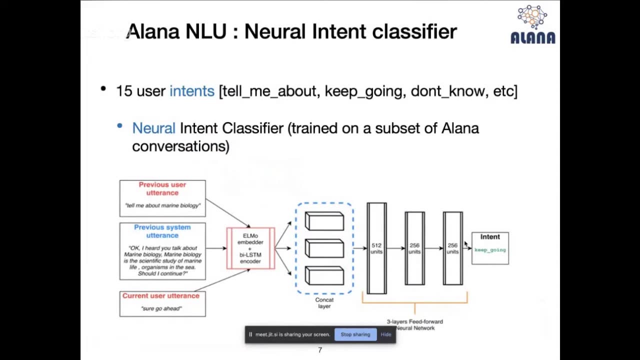 And then it has a trained in phase four, a trained intent classifier and a trained topic classifier. So this is On the next slide. This is A deep learning system that has, at the moment, 15 different user intents that we train on. 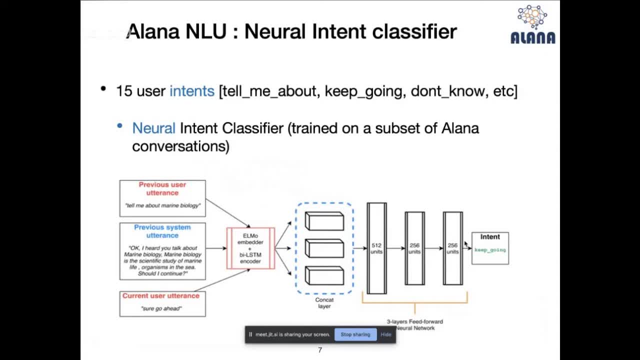 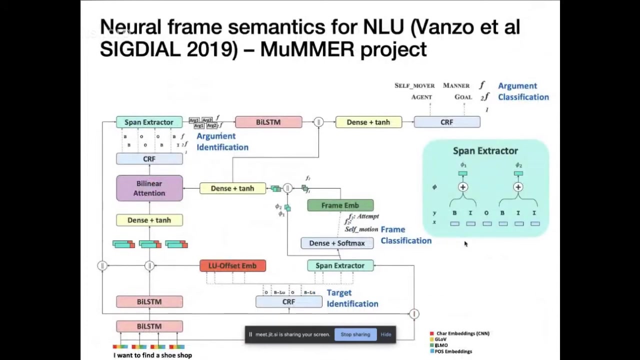 And we trained it from real data that we collected in the Alexa Prize. So we can basically upgrade that or retrain it with new data that we collect in the spring project. Another thing we did in the Mummer project was neural frame semantics, which is a slightly more complex approach to language understanding where we're able to actually derive frame semantics to representation. 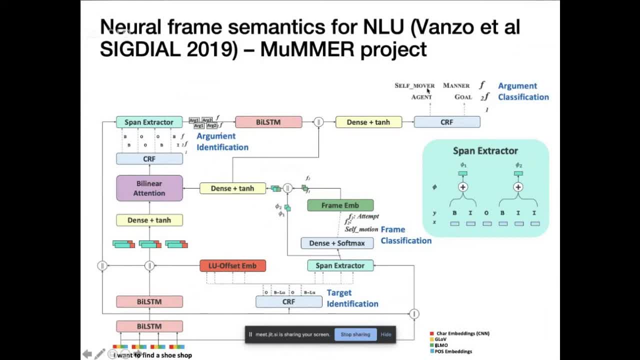 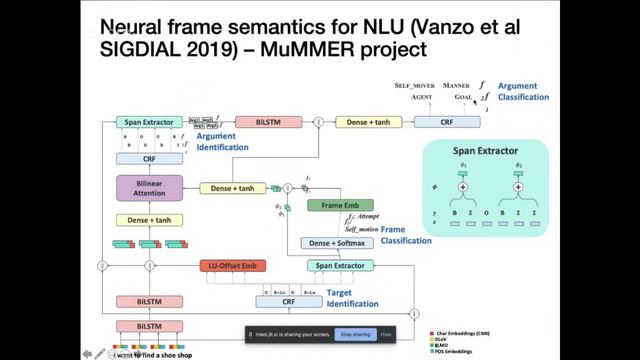 And then that sequence of words is sent through a bi-directional LSTM with various embeddings, And what we get out at the end is the most important thing. It's: We have the arguments and the frame, semantics. So we know about quite complex semantic representations. 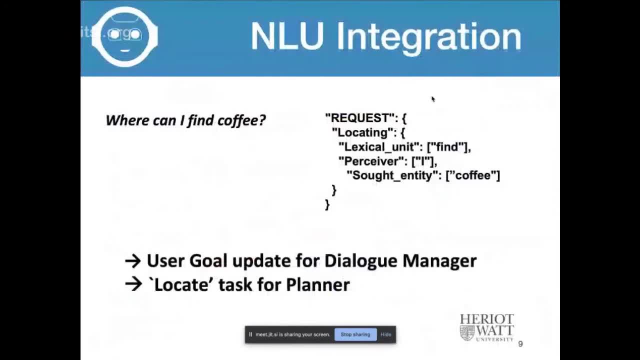 So for an example is, if somebody said where can I find coffee, We would be able to decode that into a user request to load, And then we can, of course we'll be able to find things that we want to work on. 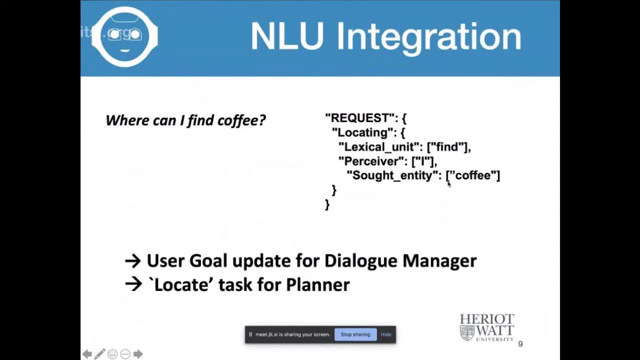 And then we can, of course, we'll be able to find things that we want to work on. So that's the first step. So the first step to locate a sort entity which is a coffee, and we even know that there's a, there's a subject, who's? 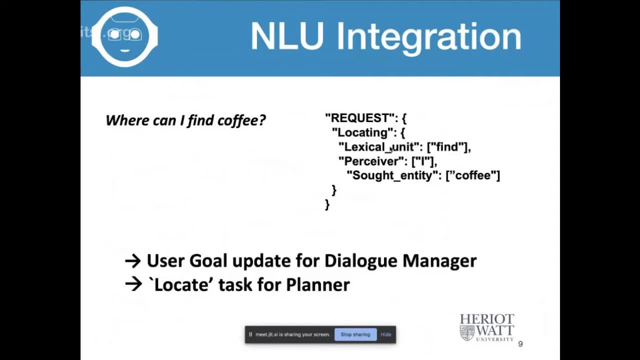 saying this, so we're able to do quite complicated semantic decoding. and then what's important is that that then updates the dialogue manager and the planner, so the user goal is updated. in this case, the user goal is to find this coffee, but also the planner is told to start doing a locate. 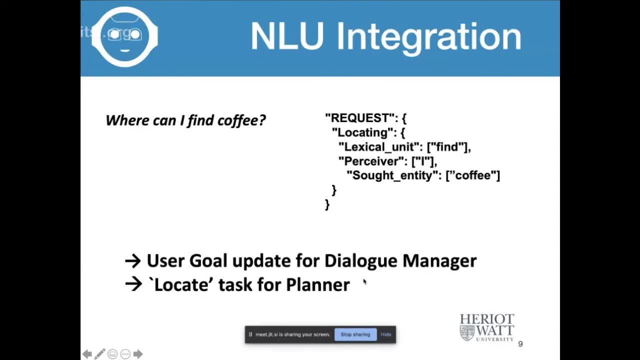 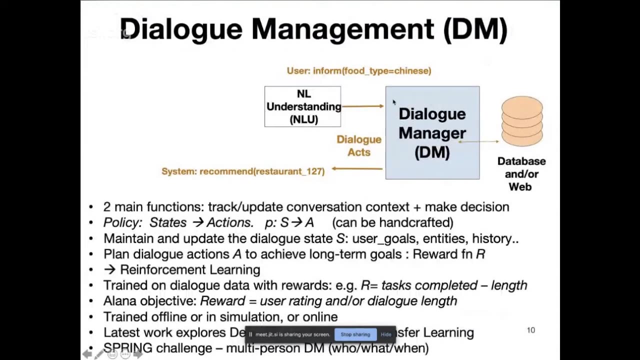 task- and that's something that christian will speak about a bit later- how the planner is integrated with the dialogue system. okay, so we're now at the point of dialogue management. um, so that is the component that's going to be responsible for um tracking the conversational context and then making decisions. 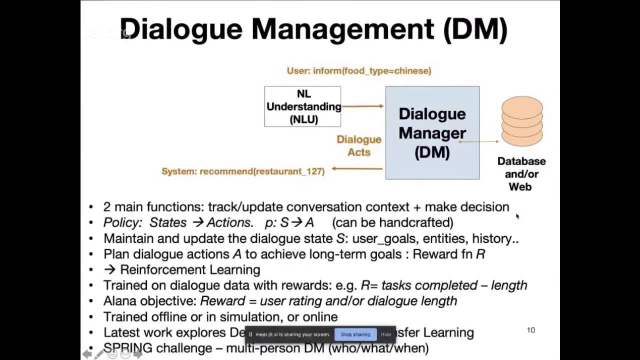 about what to do next in the conversation. so these are two very important roles that are kind of combined in this one, uh, this one component. so the way that's been represented more recently is as a reinforcement learning problem, although it can be used in a lot of different ways, but it's also in good, old-fashioned ai you would write a rule-based. 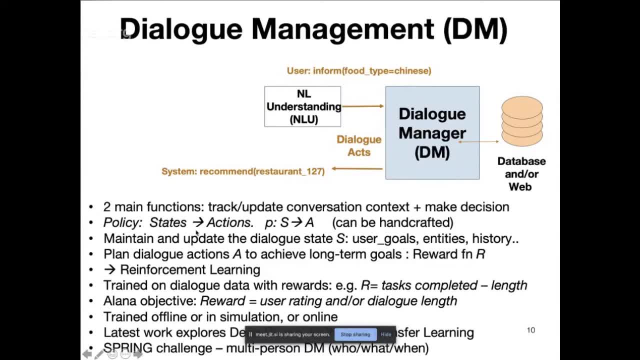 uh system to do the dialogue management, but more recently we've tried to um represent this as a as a policy learning problem. so effectively we're tracking the state of the conversation. so the state is made up of many variables, for example representing the user's goal, but also entities. 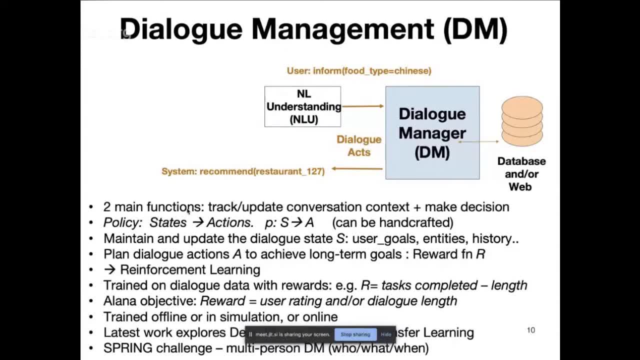 and so on and so forth. so this is a very important point that i think christian will speak about, and the problem that the dialogue manager has to has to solve is to keep the states updated correctly but then compute this action based on each state, which we call the dialogue. 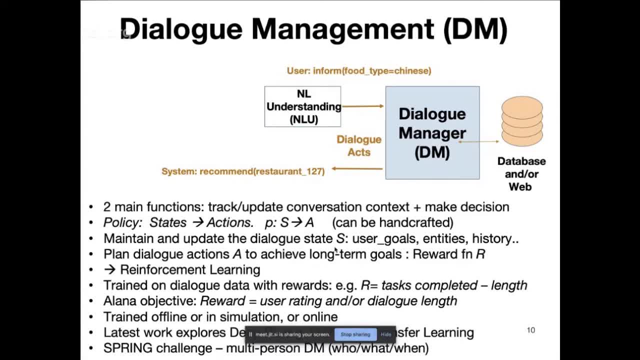 policy, um, and the dialogue policy is something um, where we're not just trying to to the user's immediate question, but that's actually a long-term planning problem, because we want to achieve long-term goals, like a long-term goal might be to recommend a restaurant. 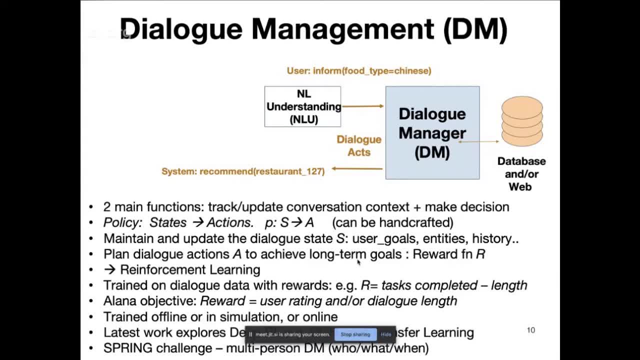 to somebody or book a flight for somebody. So we treat this as a reward function for the reinforcement learning which is usually a combination of how many tasks we've completed minus the dialogue length. So we're trying to. that basically says that we're trying to minimize the length. 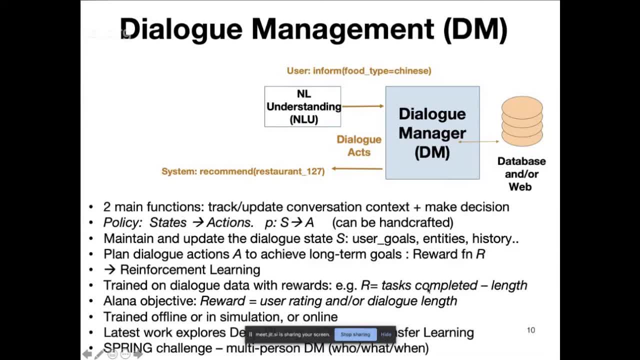 of the conversations, while maximizing the number of tasks the user has completed. So this is appropriate for task-based systems, which are where we care about efficiency. But in social dialogue, which is what the Alana system is doing, the reward is actually different. 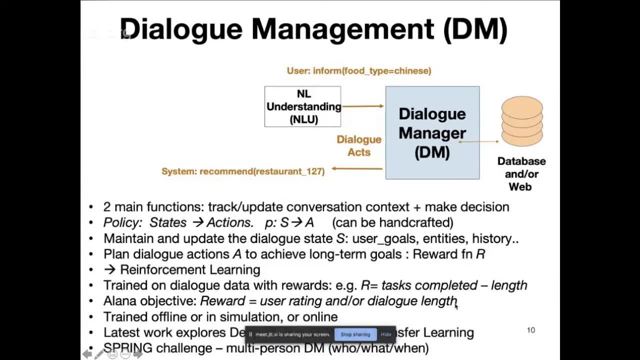 It's a combination of user ratings and the length of the dialogue, where we actually want to have longer dialogues because we're trying to engage and entertain the user. But basically the message here is that we treat this as a reinforcement, learning, optimization problem and then the dialog policy that we learn obviously depends. 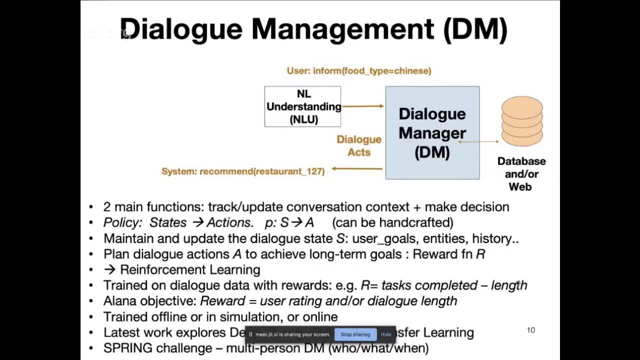 crucially on the reward function that we choose, what we choose to optimize for. So these systems are trained in three different either offline, from a huge amount of data that you've collected already, or using a simulation. So if you have an accurate, accurate, accurate, accurate, 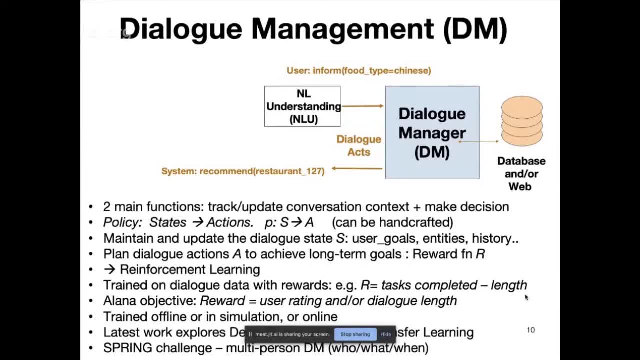 So, if you have an accurate, accurate, accurate, accurate. So if you have an accurate, accurate, accurate, accurate simulation of your user, you can train in simulation or you can train a system online in real interactions with real people. 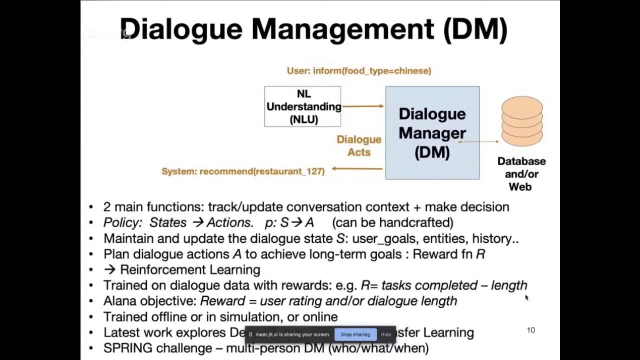 But the problem is it's very sample inefficient and you need a lot of interactions to learn a good policy And since you're learning, a lot of those interactions will be suboptimal, which is not a great user experience. Anyway, there's a lot of more recent work. 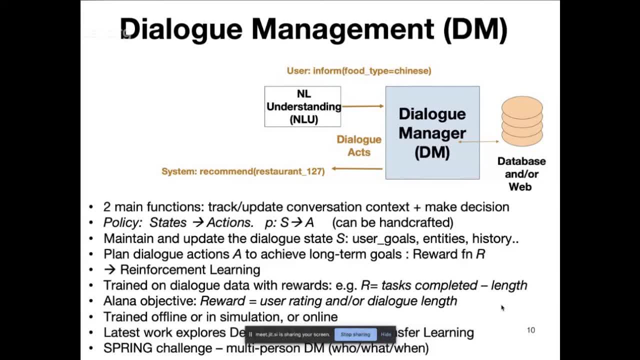 which is trying to apply deep reinforcement learning and transfer learning to this problem, And I think the interesting challenge for Spring is that we have again a multi-person situation. So who do we speak to, What do we say to that person And when do we say it? 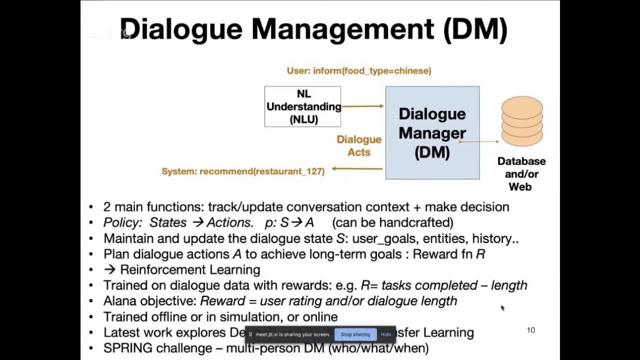 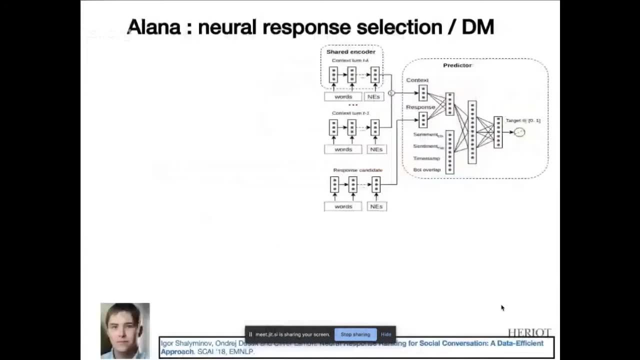 These are all now elements of the dialogue management decision in a multi-person situation that we haven't really had to deal with before. So there's a lot of opportunity for doing really interesting new work on dialogue management as well. So just to say in Alana. 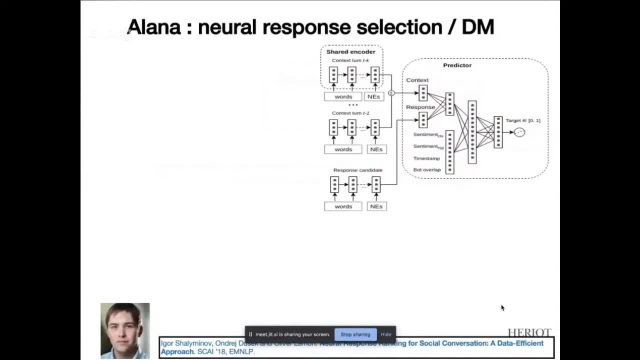 we had a deep learning set up for doing this dialog management or response selection, And I won't go into the details right now, but basically, if you're interested, you can find a paper on that. but what it was doing was learning to rank possible things the system can say next. 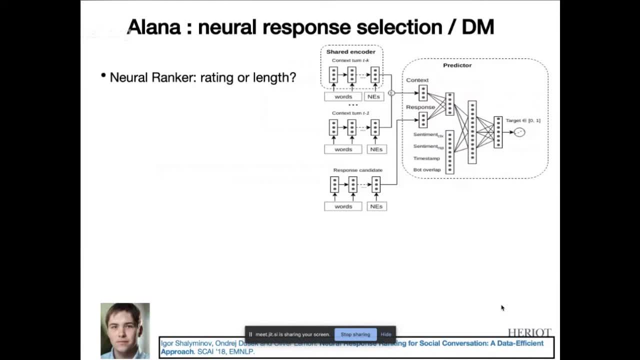 either using predicted user ratings or predicted length of the whole conversation. So we trained it on about half a million turns of data, which is a lot of data that we collected in the Alexa Prize, And we were able to build a system that was able. 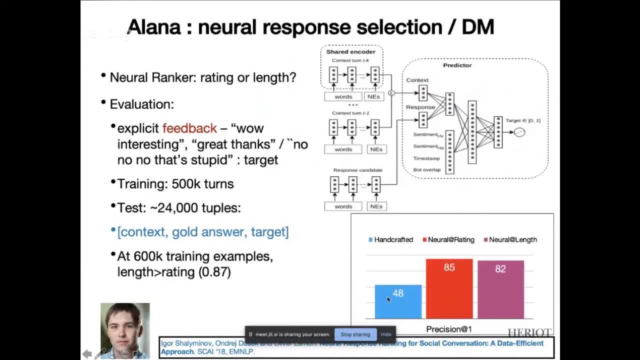 to really significantly outperform handcrafted approach to dialogue management. So the basic message here is that there are new deep learning methods for trying to figure out what's the best thing to say next in a conversation, And for Spring it's really interesting to look. 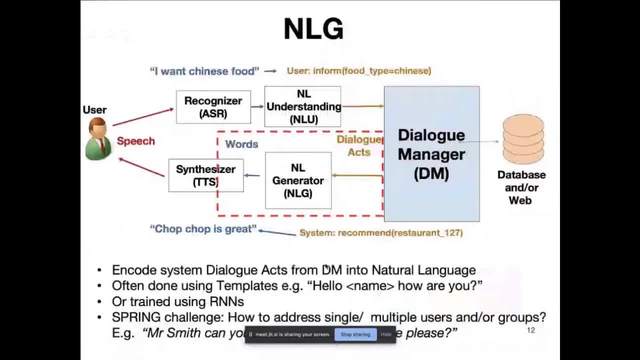 at the multi-person version of that. Okay, so that was a very rapidly growing and growing process of discussing dialogue management. Natural language generation is then the problem of encoding the dialogue acts back into a string of words of natural language. So actually most of the time, this is done using templates. 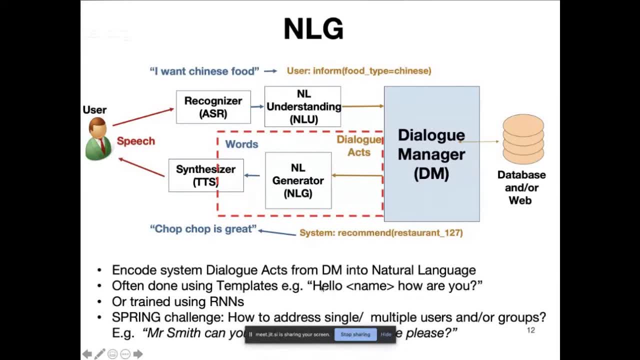 So a template is just you know. you have multiple strings like this that all convey the same kind of message and you- just you know, insert some information into that template. That's a very easy and very controllable way to do it. 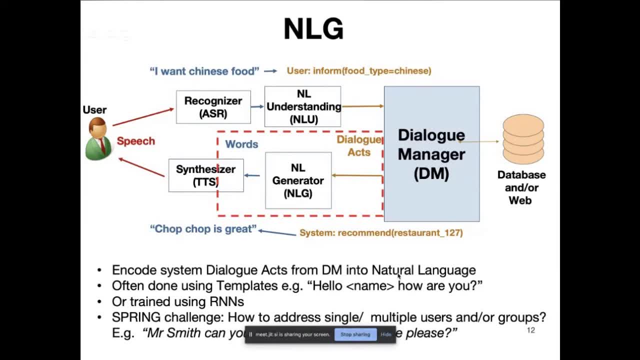 The more research oriented methods are, using again recurrent neural networks to try to train these mappings. And for Spring, again we have an interesting problem of how we address different people or even groups of people. So we have to in the natural language generation component. 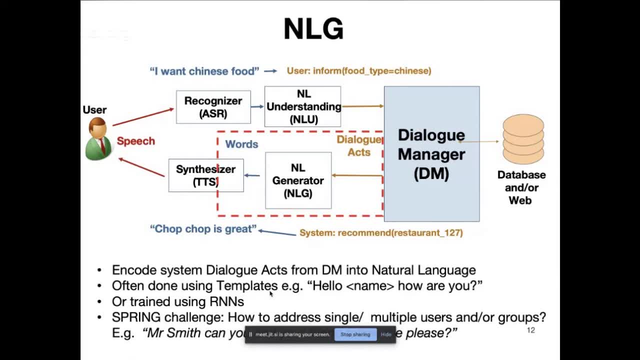 we have to maybe address people by name or even say things like you know: hey, can you two please come over here and follow me if we're addressing a group of two people. So that hasn't been done before. Okay, and then text to speech. as I mentioned before, 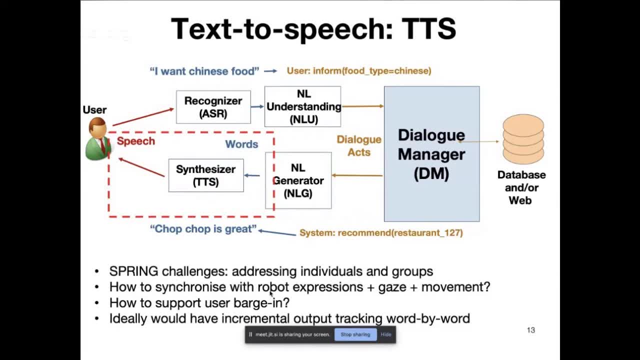 the important thing here is to synchronize the speech, Synchronize the speech output with appropriate robot gaze, robot movement, possibly even facial expressions. Also, what happens if a user barges in or interrupts the robot while the robot is speaking? What would be really nice is to have an incremental speech output. 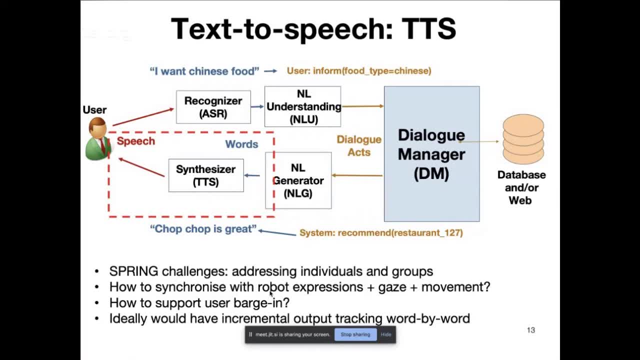 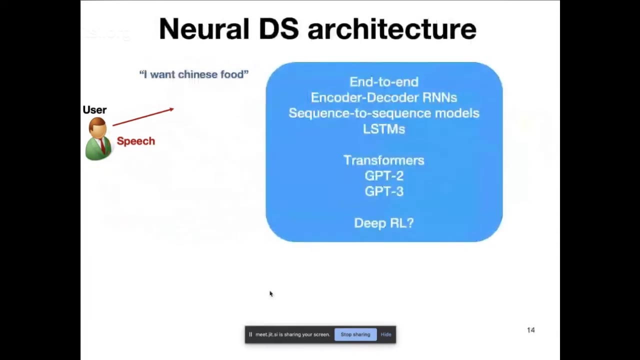 where we would know word-by-word, word-by-word what the robot is saying, And when somebody interrupts the robot, we would hopefully know at which point the robot had been interrupted. So that's an interesting problem in speech synthesis. Okay, so I mentioned earlier that actually in the modern 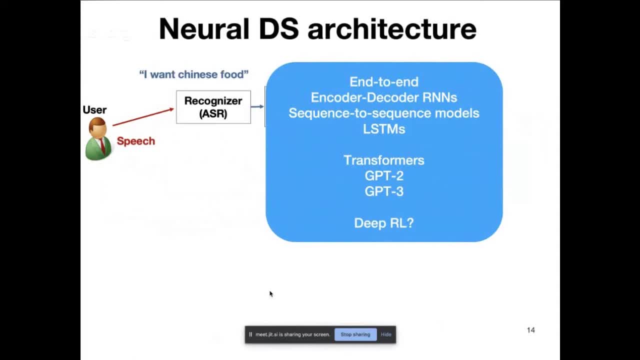 very recent work. a lot has changed And what's basically happened is that all of those components- language standing and language generation- have been to some extent replaced by these new deep learning models of various sorts, So started out with recurrent neural networks and LSTMs of various types. 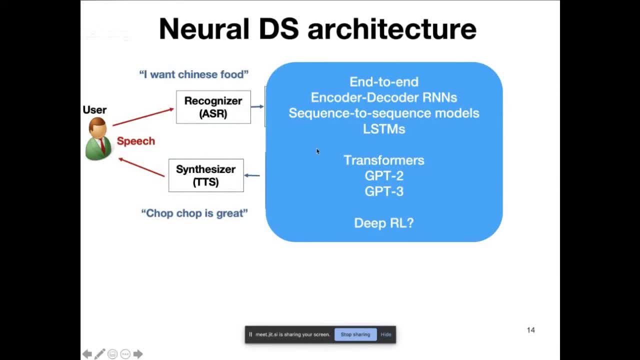 And very recently there's been a lot of work using transformers. So I think just last week GPT-3 was released And what they effectively do is learn a huge and complex language model with like millions or billions of parameters that learns to map strings to strings. 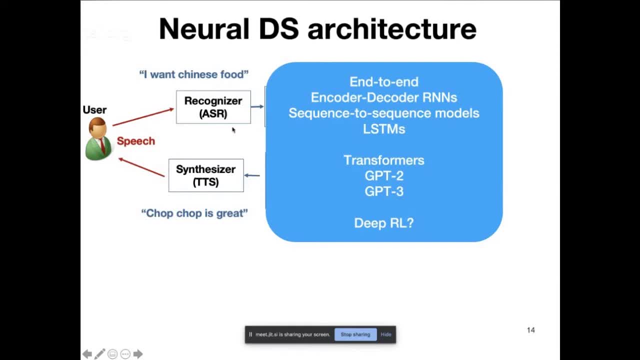 So you can do some very interesting things with these, with these methods, But the problem is that basically, this is a very large language model rather than a goal-directed interaction, And it's very difficult to condition these models on an external data source or indeed, as we need to do, on a planner or a task state. 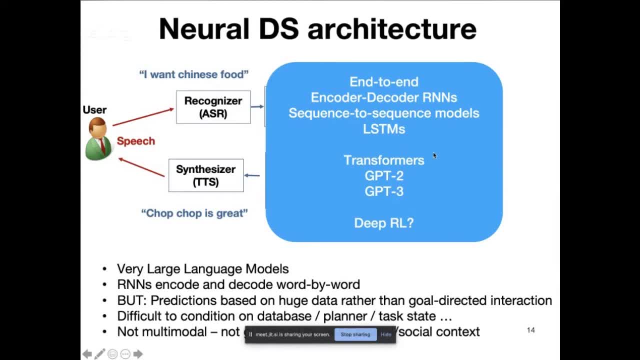 So these things are really good at kind of sort of social chit-chatting. Even then, there are still some problems with them. It's a very interesting new direction, but it's not going to be like a magic bullet for our project. 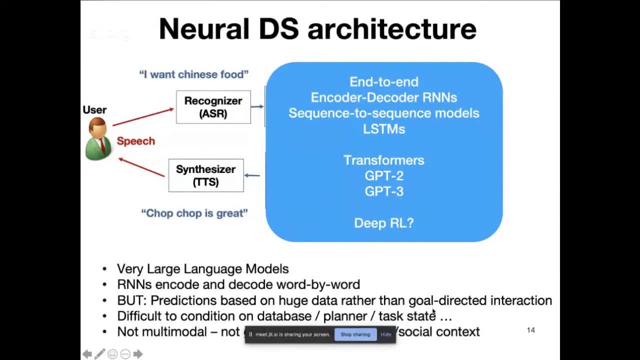 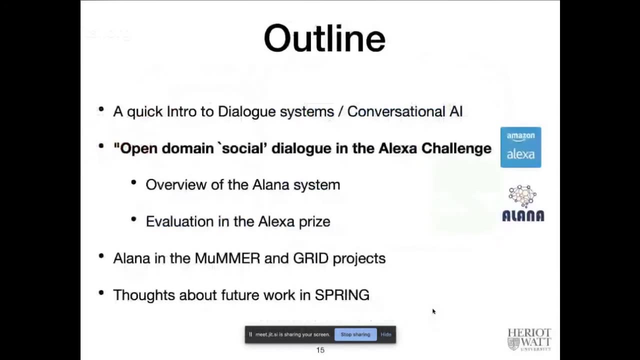 Again, they're also not multimodal. They don't have any notion of visually grounded dialogue or multi-person social context. Okay, so it looks like Christian's talk is going to have to be delayed for the next, for another session. just looking at the time. 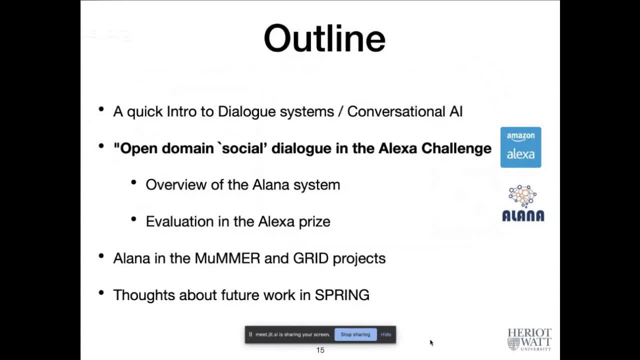 I wanted to just briefly give you an overview of the Alana system, which is kind of the foundation of what we're doing in the Spring project. So it was an open domain social dialogue system. It was developed for the Alexa challenge. So open domain basically means that you can talk about pretty much anything. 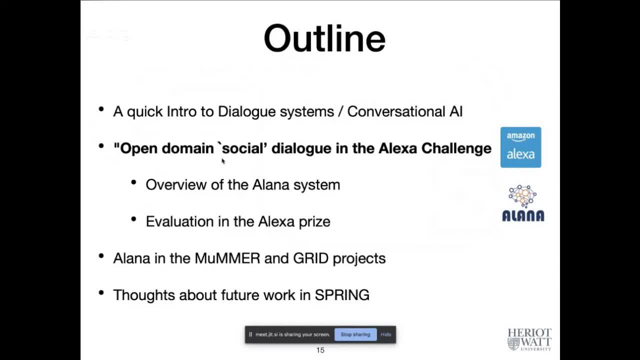 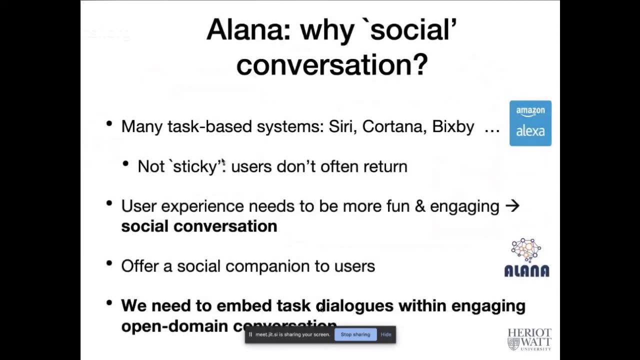 So music, movies, celebrities, philosophy, books, sports- allows the user to hopefully talk about whatever they're interested in. The reason this is interesting is that there are lots of task-based systems like Siri and so on, But the problem with them is that people don't often really talk to them very much. 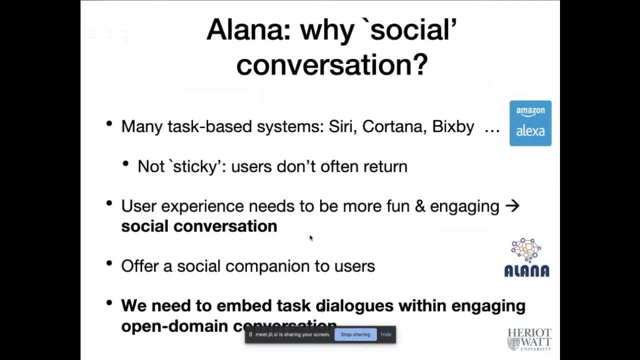 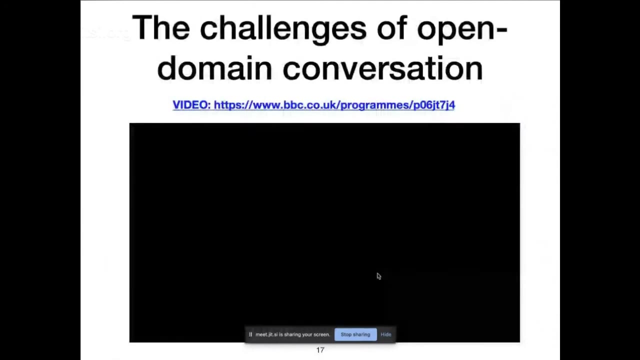 They're not very fun or engaging And they don't really offer the kind of social companionship that, ultimately, we would really like to develop with these kind of personal assistants. So what we want to do is embed task-based conversation inside a much more engaging, social, open domain conversation. 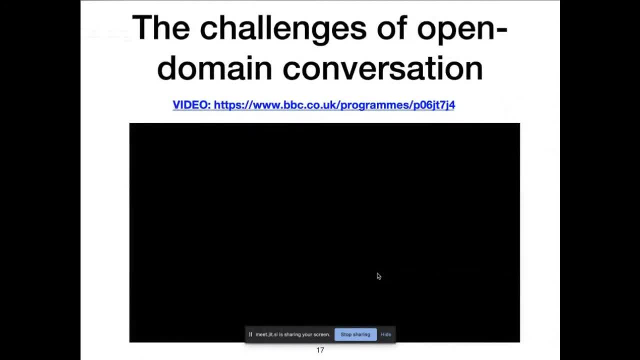 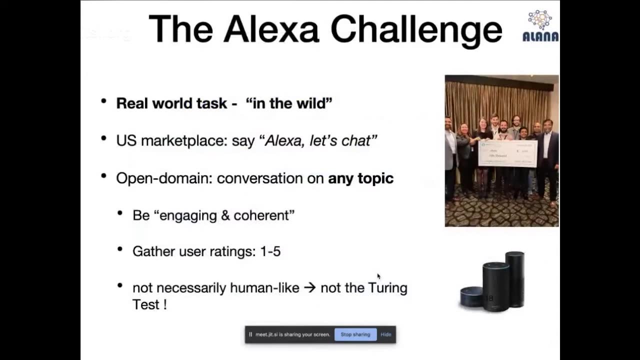 So you can watch this video at your leisure. I'm not going to show the video now, But it's a video demo of our system a few years ago from the BBC Okay. so it was released to the whole North American marketplace for two years. 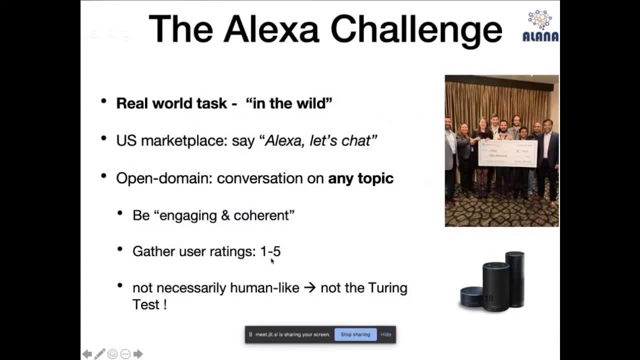 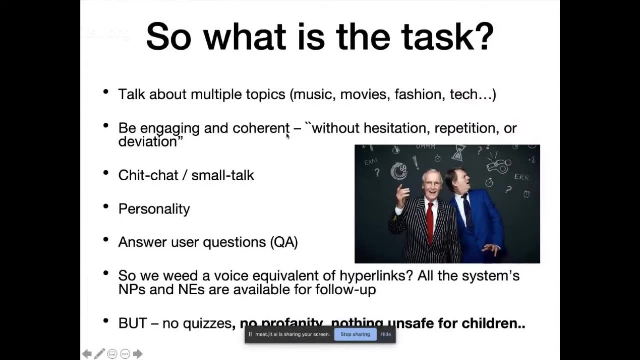 And we gathered a lot of user ratings, So people could give a rating between one and five stars And, as I said, the task is to talk about lots of topics- music and movies, and fashion, whatever- And to try to do that in a very engaging way. 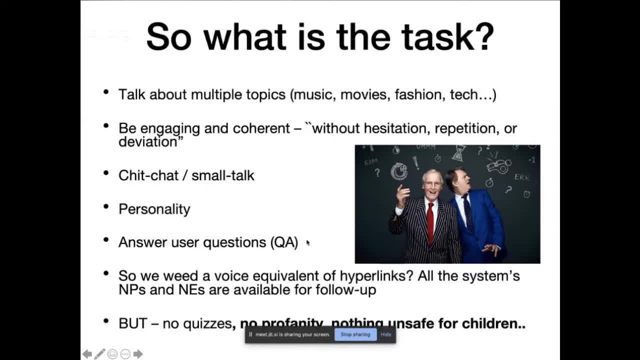 together with some personality, Also answer people's questions. So it's a really very challenging AI problem And another important facet of it is kind of ethical issues: That you can't give people information that's sort of unsafe for children or could offend people. 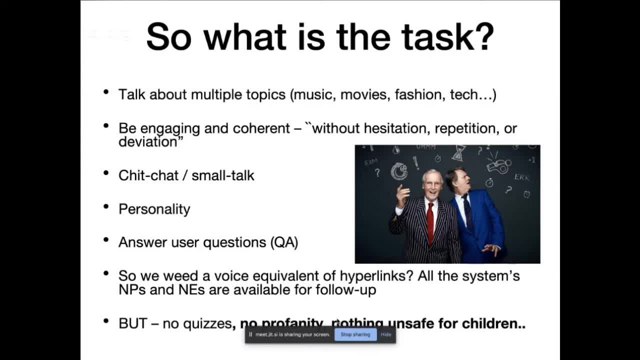 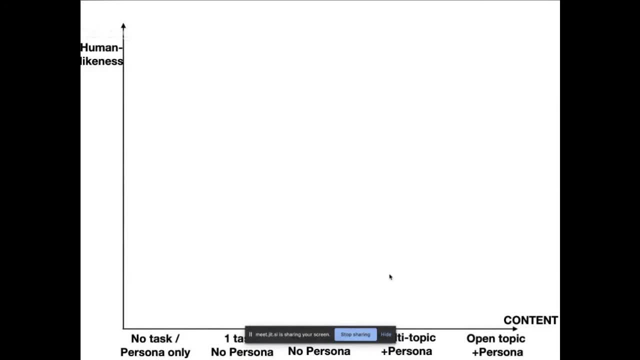 So you can't just grab any old information off the internet. So here's a kind of graph that tries to represent where these systems live on, a kind of in the landscape of different types of dialogue systems. So if we look on the y-axis, I've got human-likeness. 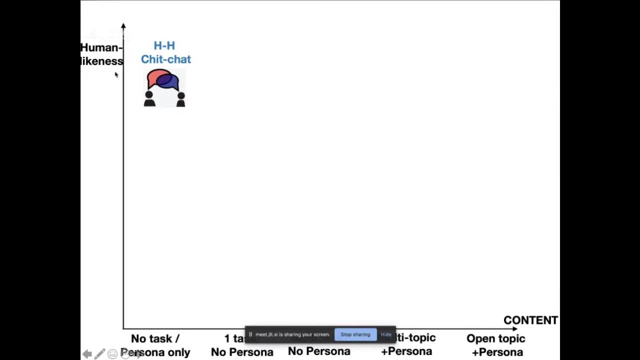 So how human-like is a system? So human-human chit-chat is where we are not talking about any task And it's just about personas or personalities, And humans are the ultimate chatters at that. So on the x-axis I've got different types of systems. 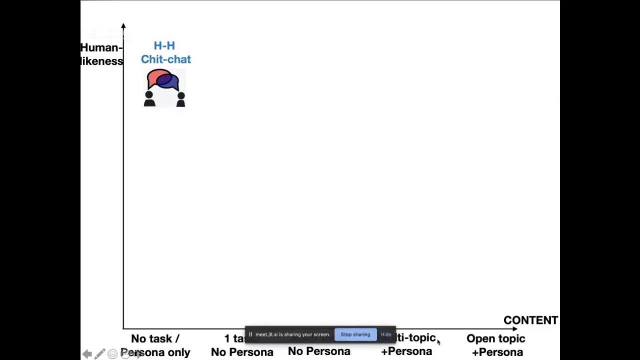 If you don't care about personality, you're just doing tasks, Or you want to talk about multiple topics with a person. So this is kind of how complex the content is getting on the x-axis. Okay, so we have human call center operators. 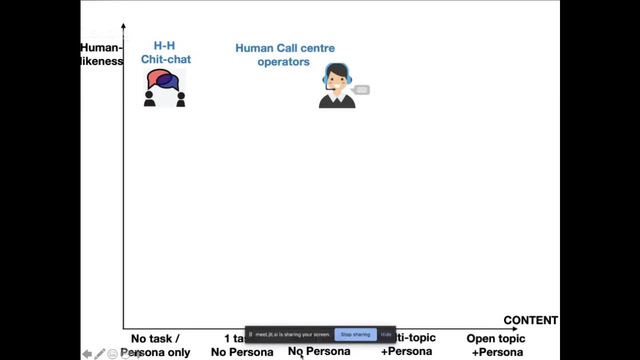 They're really doing tasks where they're not really having a persona other than being trustworthy Humans or anything that passes the Turing test would be up here, where we can talk about multiple topics with a personality. So there's an old system called ELISA, which you may have heard of. 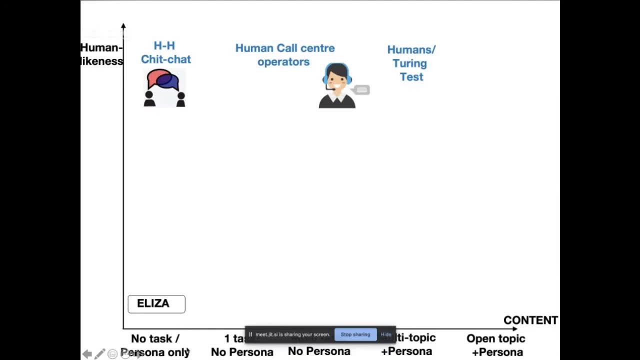 which was not very human-like, But it was kind of a sociotherapist bot. It lives down here. All of these new language model-based systems live around here. They are doing chit-chat but they're not doing tasks And they're not quite a human performance. 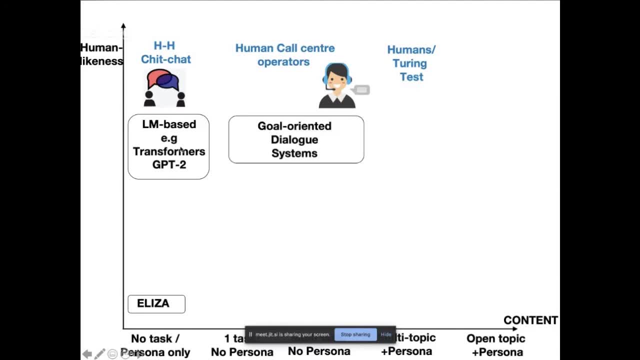 but they're pretty human-like in some ways. Then there was a whole load of research on goal-oriented dialogue systems over the past 20 years And it lives around here. There's lots of work on chatbot. that is really spanning a huge range of different types of scenario. 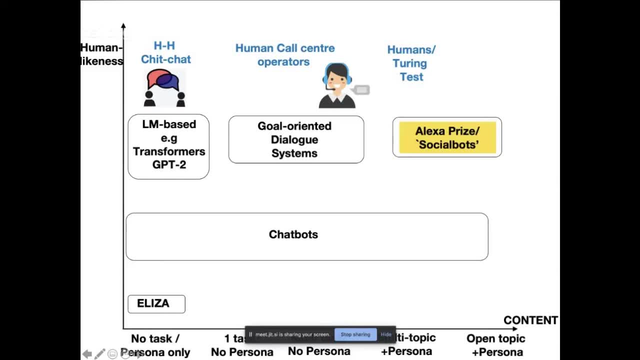 but it's still not very human-like. And then the Alexa Prize social bots are somewhere in this region where we're doing multi-topic conversation with personality And we're trying to begin a conversation to become as human-like as possible. So this is just trying to give you a little bit of an idea. 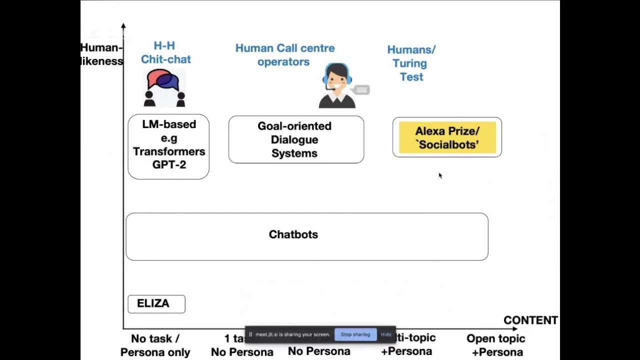 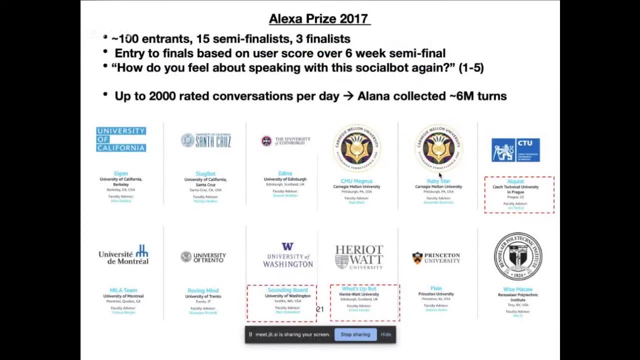 of the different types of system that are being developed. Okay, so we entered the prize for two years And, in a nutshell, we were finalists for two years, But, more importantly for us, we collected about 6 million interactions with the system. 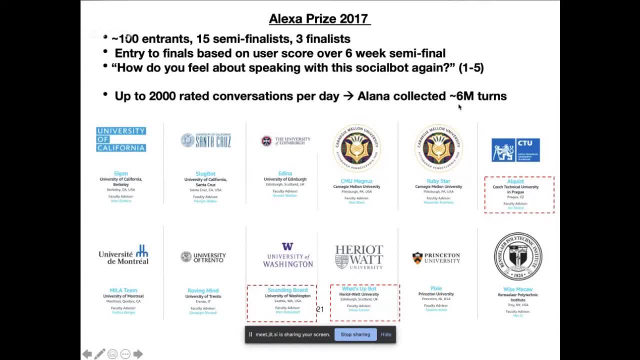 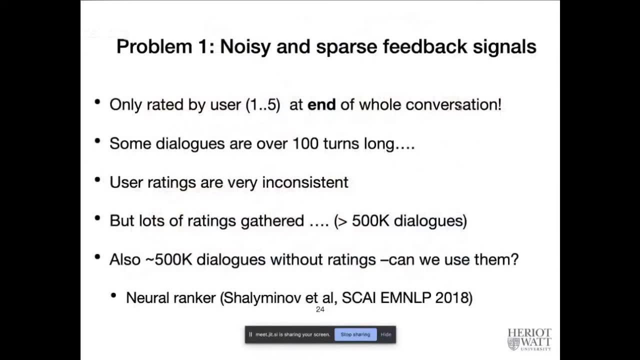 which is a huge and wonderful amount of data to train systems on. I'll just zoom through. So from a scientific point of view, the interesting problems are that we have a very noisy and sparse feedback signal for training the system, So users only rate the system at the end of a whole conversation. 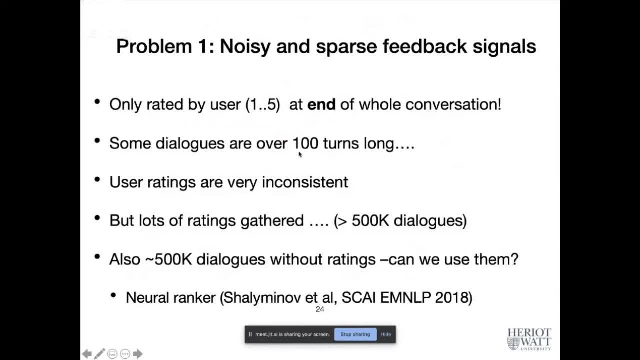 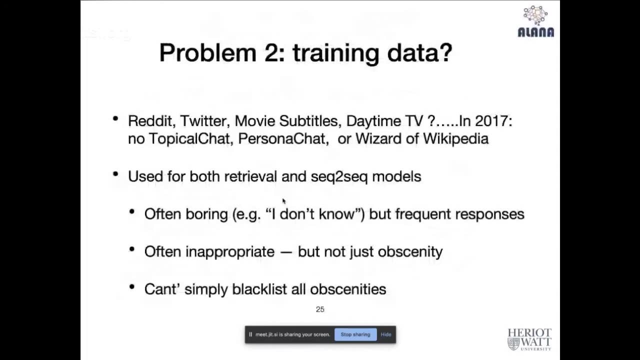 Some of these conversations are hundreds of turns long, so it's a very weak reward signal for training. So we still were able to use them in that deep learning neural rancor that I mentioned earlier. The other problem, main problem, is how do you get data to train this kind of system on? 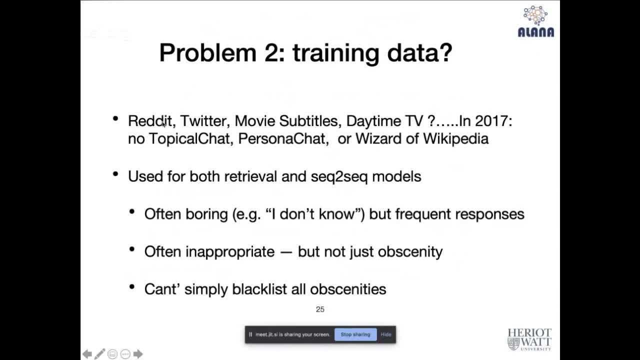 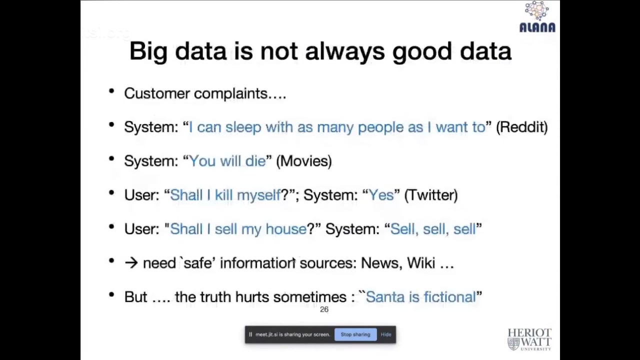 So we actually used initially data from Reddit and Twitter and movie subtitles and even daytime TV shows. But we ran into some serious problems with this. Basically, the system was producing very inappropriate outputs. So here's some examples. If you train on Reddit, 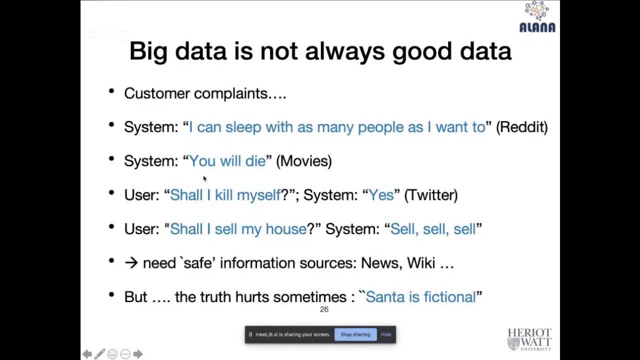 your system will say things like this: If you train on movie subtitles, it will say things like: you will die. So you really need to control the information sources of such a system. So what we settled on in the end is basically having safe information. 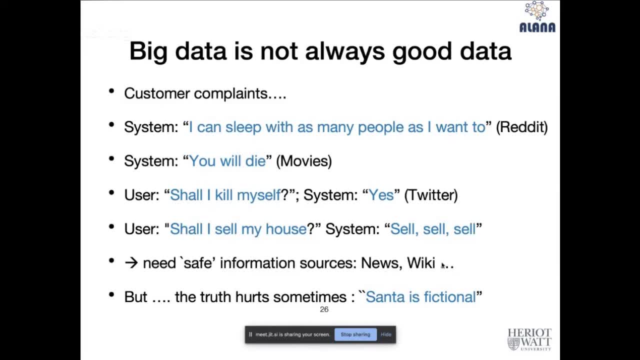 from Wikipedia and from newspapers. Even then we still run into some problems. So we actually had a mother complaining that we told their child that Santa is not a real person. So Amazon really cares about this kind of thing because they don't like user complaints. 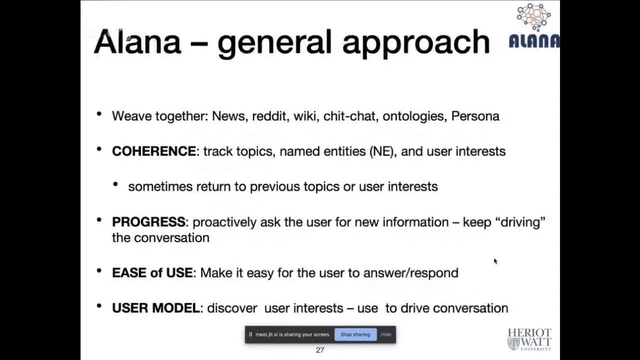 Okay, so Alana basically is weaving together lots of different information sources like newspapers, a safe area of Reddit, Wikipedia. We also have some ontology information about entities in there, And what we basically try to do is to track the topics and the named entities. 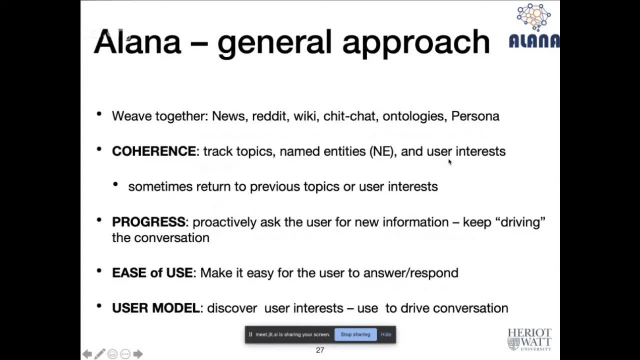 that people are speaking about, as well as the interests of a particular user. So we have a user model which is persistent over different conversations. So we remember that somebody's interested in, say, science fiction movies, And then another principle is that we always keep driving the conversation forward. 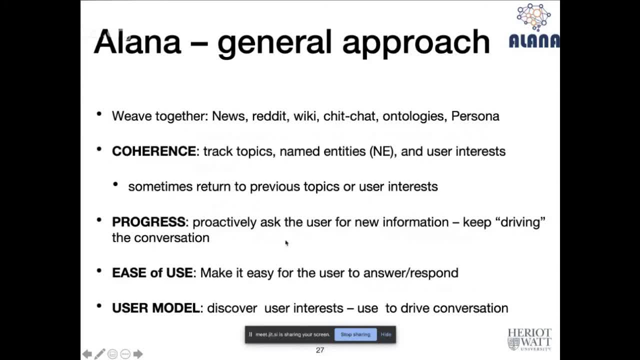 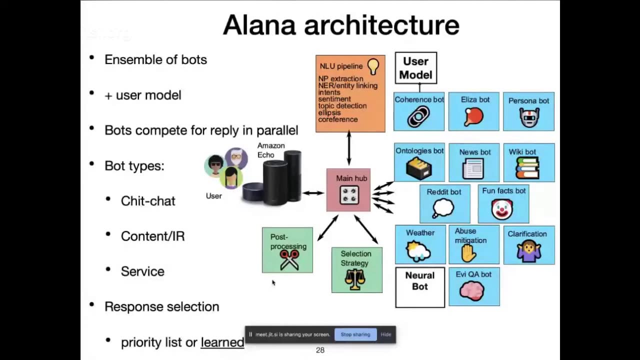 getting the user and proactively asking the user what they're interested in, what they want to talk about. We make it easy for the user to answer questions and so on. So the system we've got is what's called an ensemble system. Ensemble just means it's a collection. 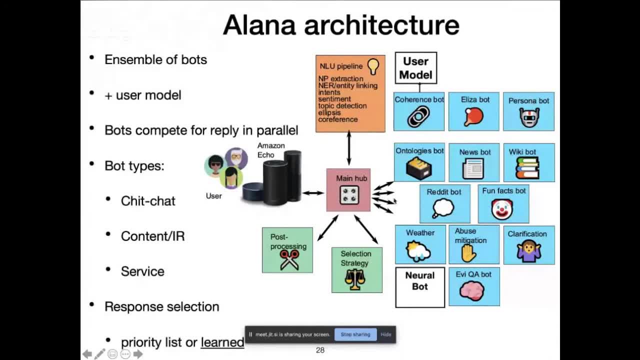 of different bots. So here on the right-hand side in the blue you can see all the different bots that make up a lot of the system, And then on the left-hand side you can see the bots that make up Alana. So we have a Wikipedia bot. 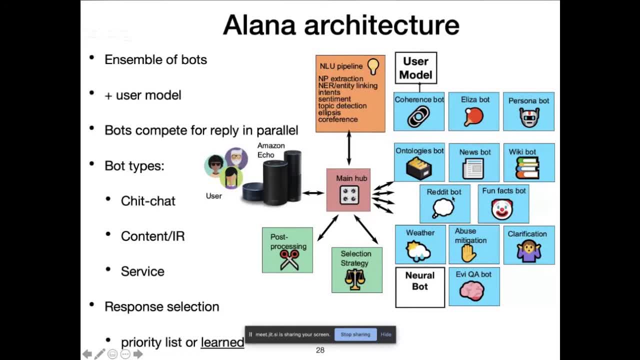 a news bot, the personality We have a Reddit, something trained on Reddit, something that knows about fun facts, all of these different types of information source And basically what's happening is when the user speaks, either to Amazon, Echo, but also we've deployed this on Google Actions. 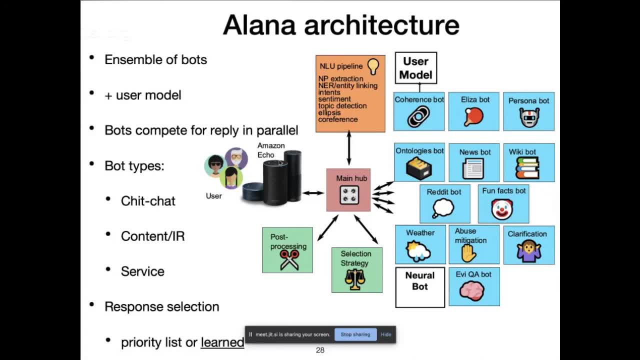 on Android phones as well, or it can be a text. We also, obviously, we deployed it on the Pepper robot as well. The user speech is decoded by a recognizer and then it goes through this language understanding pipeline that I mentioned briefly before. So we extract a lot of information. 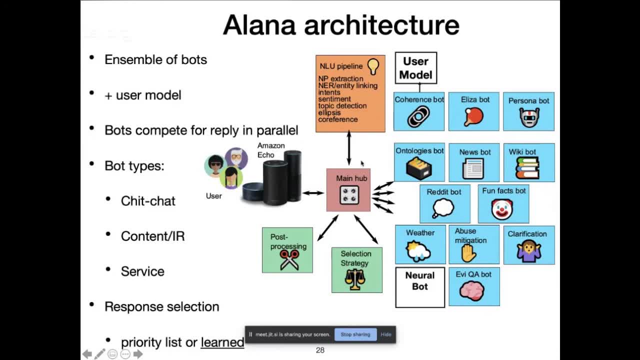 from the user speech. We put that into the dialogue context and then all of these different bots potentially can suggest something that should be said next in the conversation. And then the problem we have is to rank the different bot outputs and select the best thing to say. 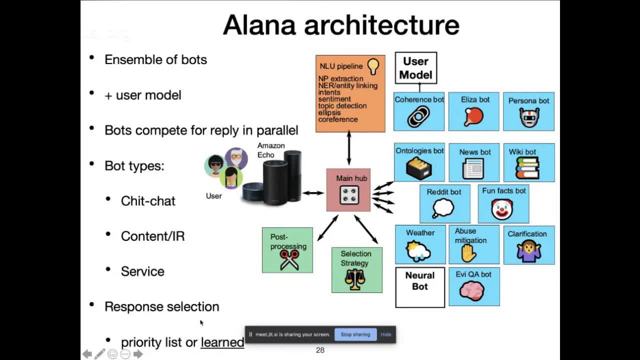 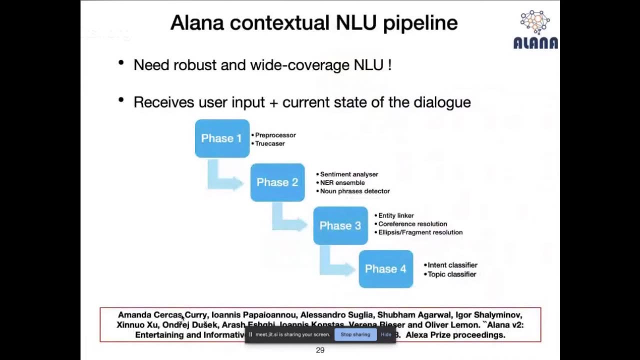 in any situation, hopefully. So, as I mentioned earlier, we actually have a learned policy for doing that, that utterance selection. Okay, I've shown this slide before. That's just about how to extract the user intents from the user speech. 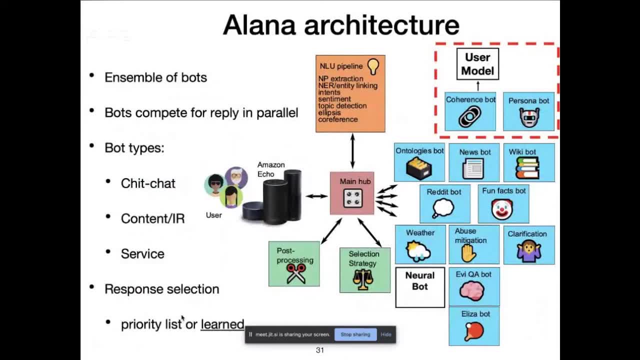 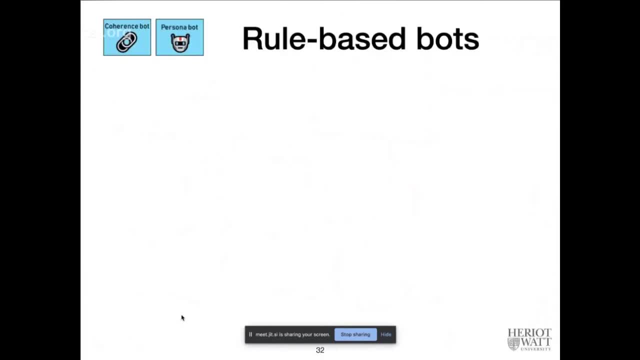 Let me see how much time I've got, Maybe five minutes left or so on. I'm just going to skip through, hopefully to more interesting parts. So yeah, so I think some of the most interesting stuff is on information retrieval. So what we have there is an ontology. 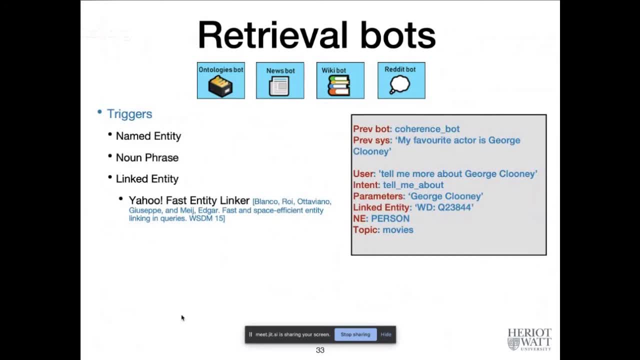 that's able to use linked data. So, for example, if someone says their favorite actor is George Clooney, we are able to extract the entity George Clooney. We find an entity in Wikidata, We know that it's a person and the topic related to this person. 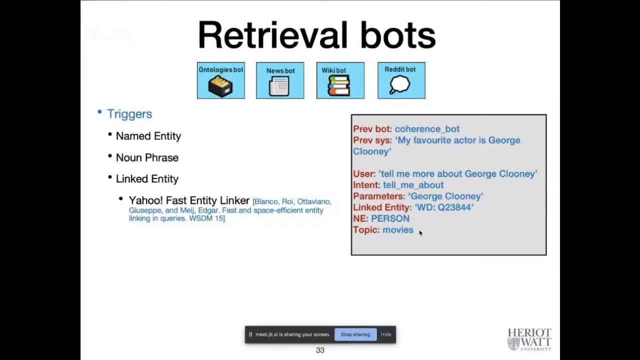 is a movie's topic And we can also look at people linked to George Clooney, So that enables or movies that he's been in, this kind of stuff That enables us to talk about more interesting news stories involving him, and so on. 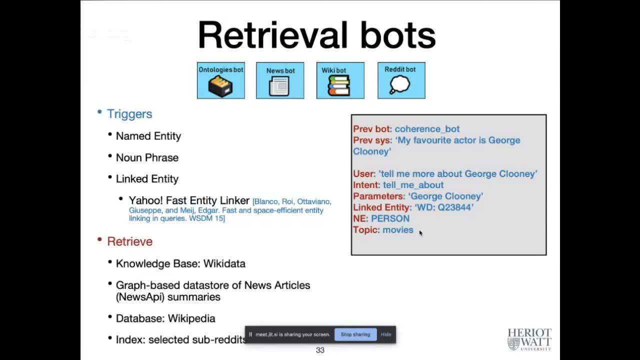 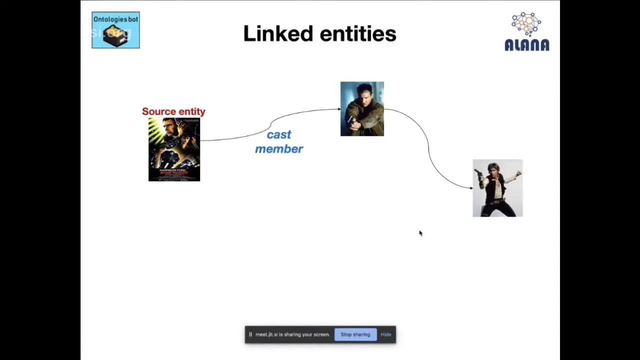 So a lot of the interesting conversation we have is using this linked data property. So yeah, so, for example, we can see that Harrison Ford was in Blade Runner, but also in Star Wars, And we can come up with even just using templates. 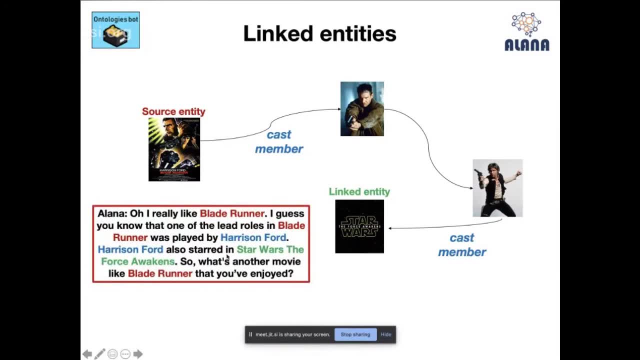 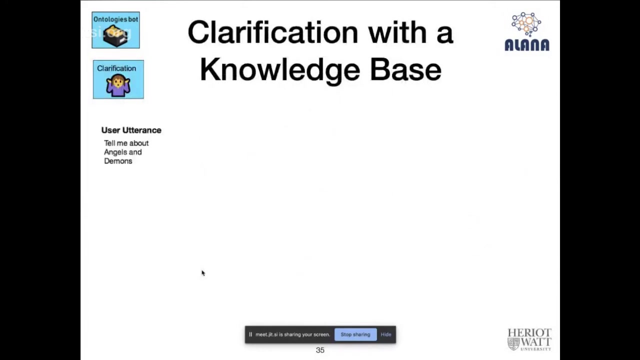 we can come up with these kind of quite rich outputs that offer a lot of information to the user, but also then ask them to push the conversation forward, ask them for more information. It also enables us to do clarification of various types. So you know. 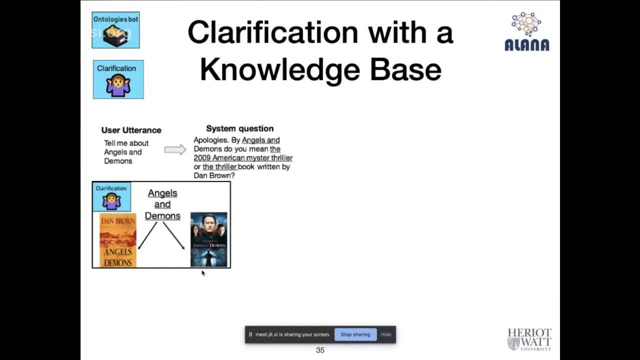 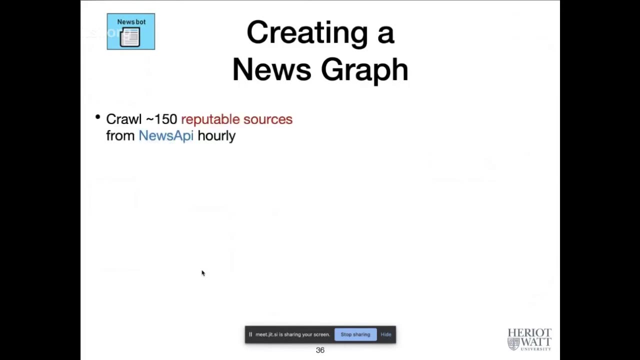 if something is both a book and a movie, we can detect that using the ontology and then do clarification of different types, And we apply similar techniques in the news graph. So every hour we compile a graph from 150 different newspapers and we summarize the stories. 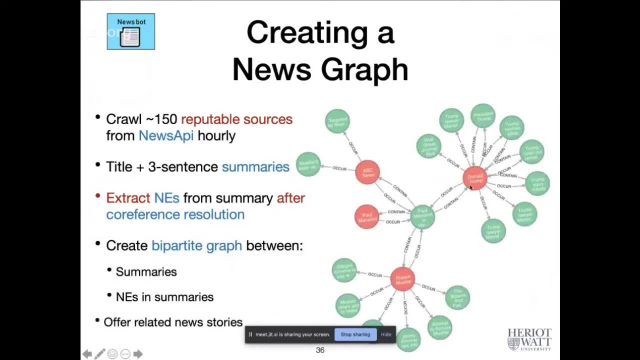 And then you're able to do things. like you know, if someone's talking about Donald Trump, then we can say, oh, related to Donald Trump, there's a story about Robert Mueller, Would you like to hear about that? So we're able to sort of offer. 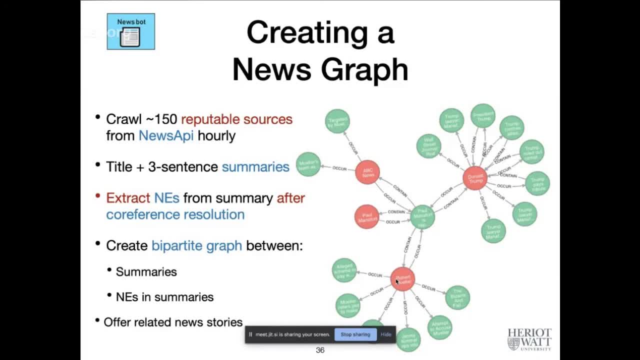 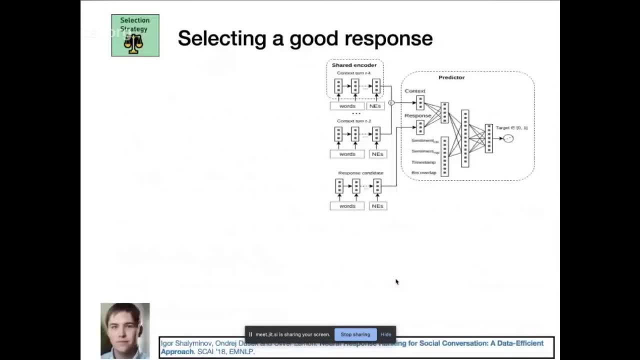 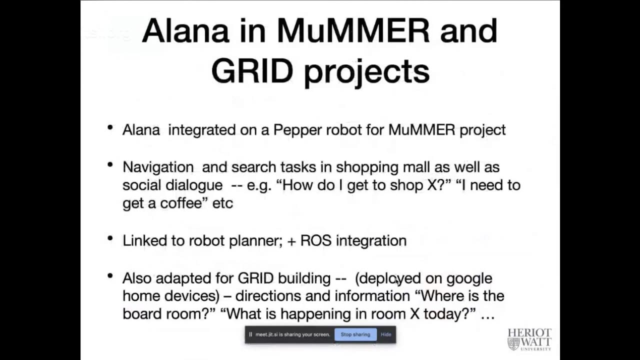 this kind of information browsing capability. Okay, And I'm just. I think I've already spoken about how we do utterance selection, at least very briefly. So it was at this point that I was going to hand over to Christian and allow Christian to speak. 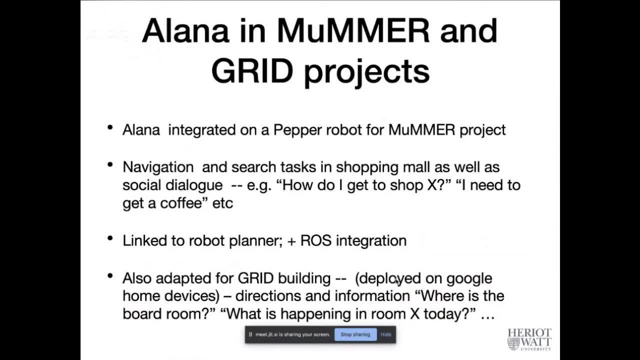 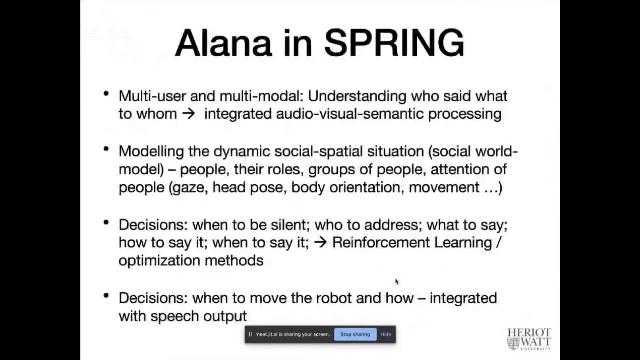 But I won't be able to do it. No, no. So how about I will, just then? sorry about that. I'm just going to very briefly talk about this last slide, then, which is what I think about Alana doing in the spring project. 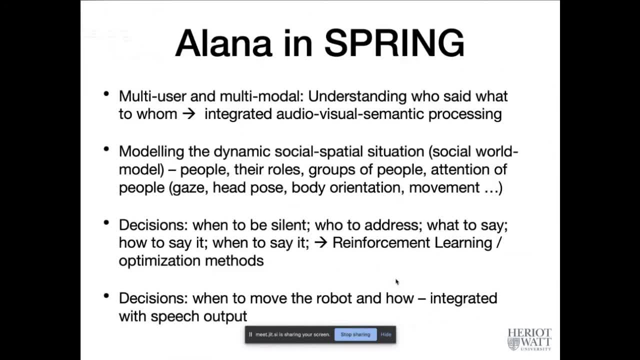 I think a lot of this we've probably covered briefly already. So, as I said, we're now in a multi-user and multimodal situation, So we have to understand who said what To whom. So we've spoken about that earlier. We want to model this dynamic. 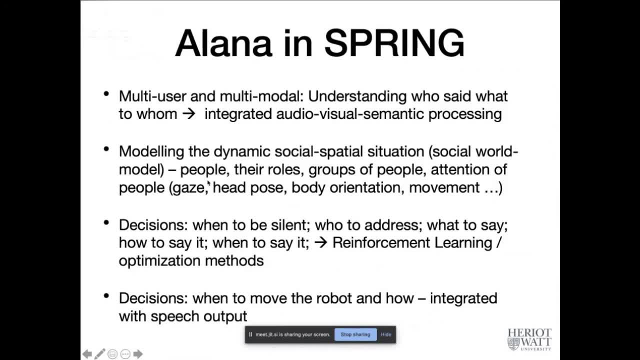 social and spatial situation, So people, their roles that they have in a particular scenario, maybe even groups of people, and their attention. And then, from a Dalai Manchin point of view, there are these decisions like: when should I be silent and just listen? 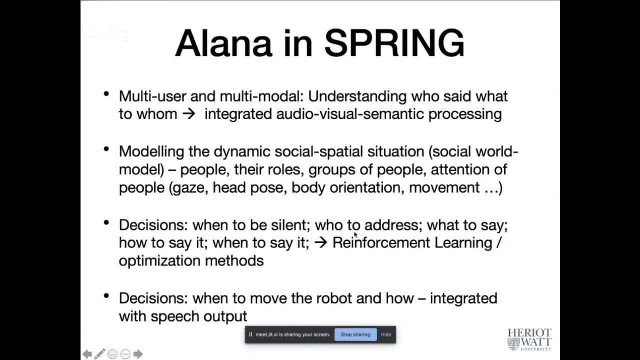 When should the robot talk and who should it talk to? So I think there's a very interesting problem in reinforcement learning of the dialogue manager for the spring robots. And then, when should we move the robot? When should it point to people or look at people? 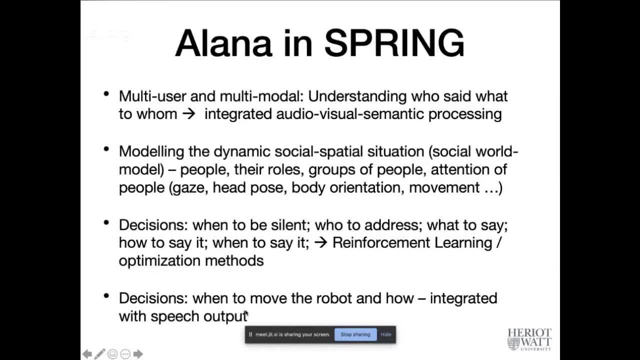 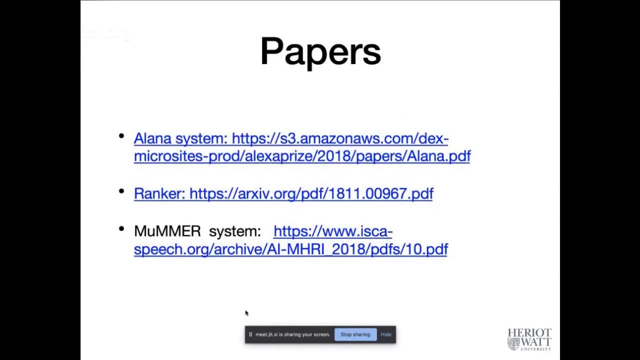 And how is this integrated with the speech output? So those are just some of the some of the very interesting things I think we can work on in the spring, The spring project, Yeah, And then at the end of the slides you'll find some papers that link.